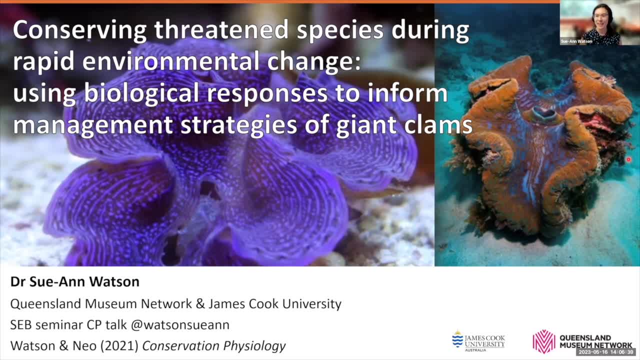 tried to keep some of the examples kind of eco-physiology focused maybe, rather than some of those field-based studies. But all the information is in the paper so you can always refer back to that if you need to. So I pre-recorded this talk for you today while I'm at the university. 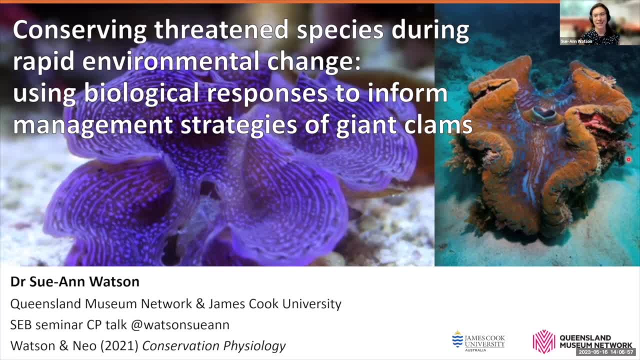 because our internet at home- we live just outside of Townsville in Queensland, Australia- can be a little bit patchy, So I pre-recorded it while I'm at university today and I'm going to be online with you after for the Q&A session. 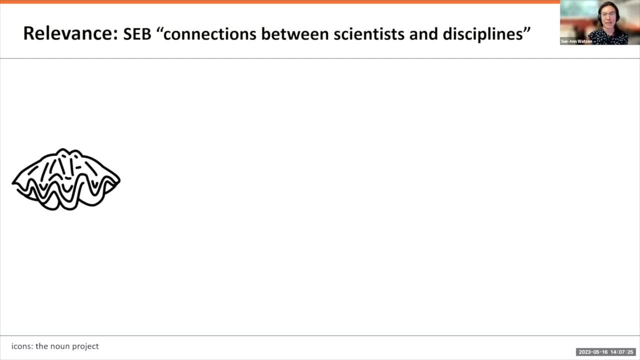 So I just wanted to start a bit about the relevance. Obviously, this talk is going to be about giant clams, but I also know that the Society of Experimental Biology really favours those scientists and disciplines. So what I thought would be good for you to think about during this: 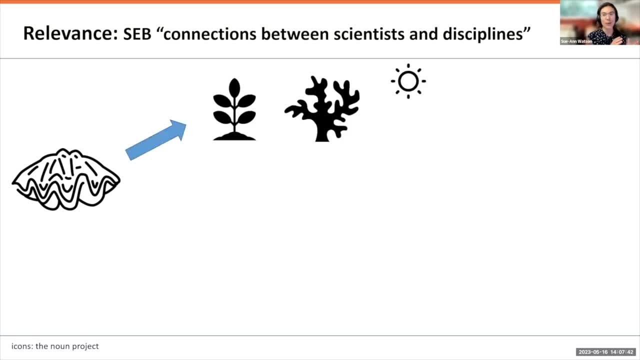 talk is about giant clams, but also how they can relate to other organisms that use solar energy- and I'll talk more about giant clams being solar powered later on- such as that animals like plants and corals, And also how this might relate to other threatened species that you may work on. So I've 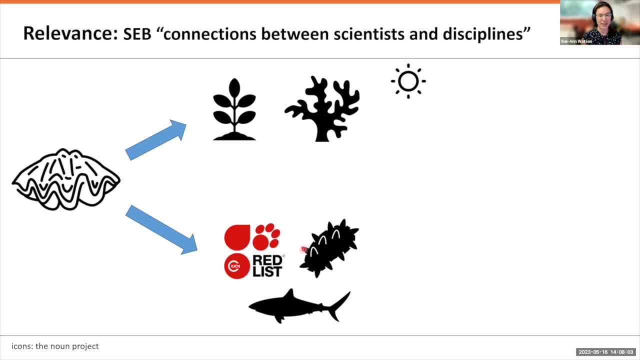 got sea cucumber Iquan here- Thank you get the pointer- and and also other threatened species and kind of the combination of both. so those species that might be threatened are soil powered and we don't know about the their vulnerability yet, so perhaps they're even yet to be accessed. instead, in terms of their extinction risk, 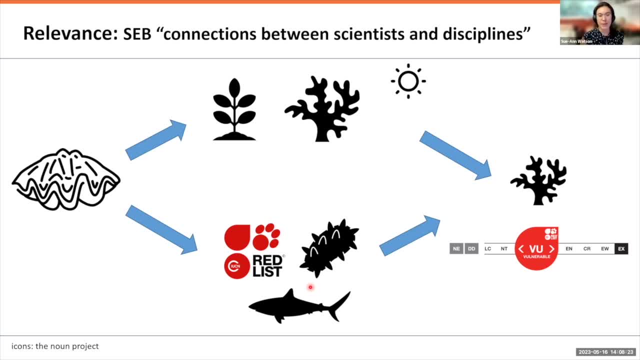 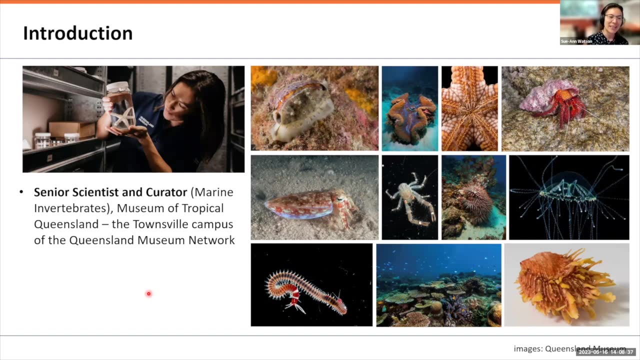 so perhaps some of those things to think about as we go through the talk. and I've also introduced a little bit of background about myself, so my name obviously is Sue-Ann Watson, so I'm a senior scientist and curator of marine invertebrates at the Museum. 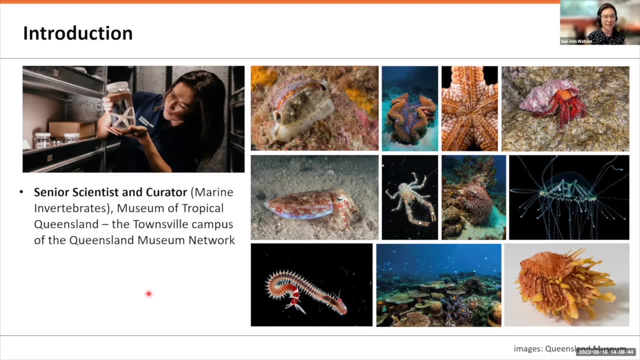 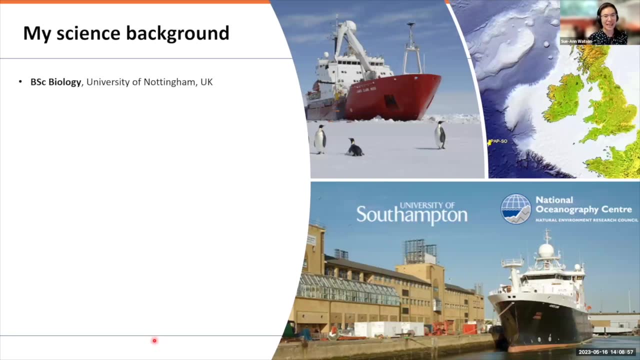 of Tropical Queensland, which is the Townsville campus of the Queensland Museum Network. I also work at James Cook University as a senior lecturer. so, in case you haven't met with me, I'm Sue-Ann Watson and I'm a senior lecturer. so before, my science background is: I'm originally from the UK, where I studied biology. 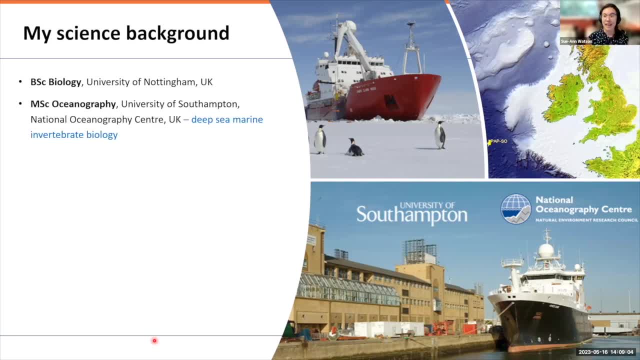 and then I moved to Southampton to study a master's in oceanography, where I worked on deep sea marine invertebrates. I continued at Southampton for a PhD, where I also worked with the British Antarctic Survey investigating eco-physiology in polar and temperate marine invertebrates. 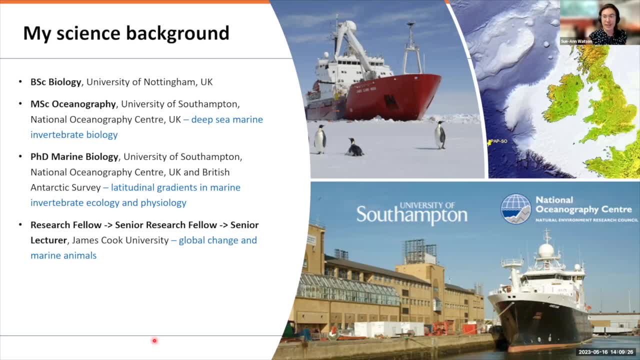 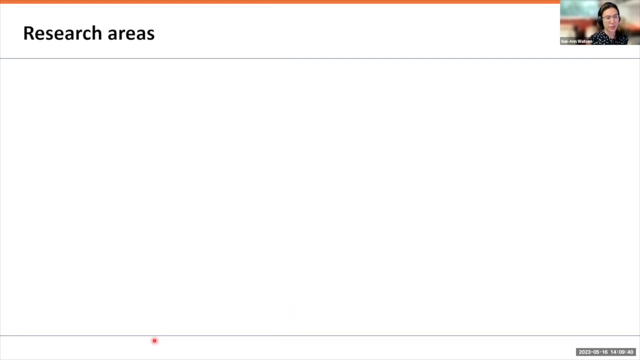 and I came to James Cook University as a research fellow and then now a lecturer, as I mentioned, and I also have that job with the museum and so kind of incorporating both of those positions. now the research that we do in our group tends to be focused on the responses of marine organisms. 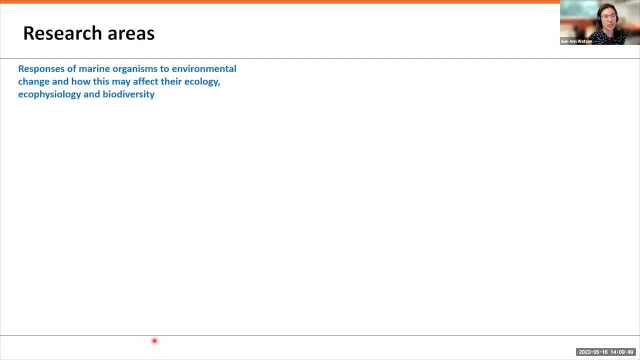 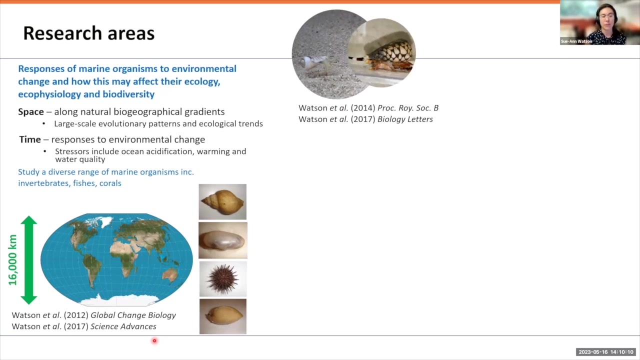 to environmental change and how this might affect their ecology, eco-physiology and biodiversity. so we tend to focus on change through space. so this might be a long natural biogeographical gradient, such as latitude- and there's a couple of examples of research here- and also change through times that could be responses to environmental change. 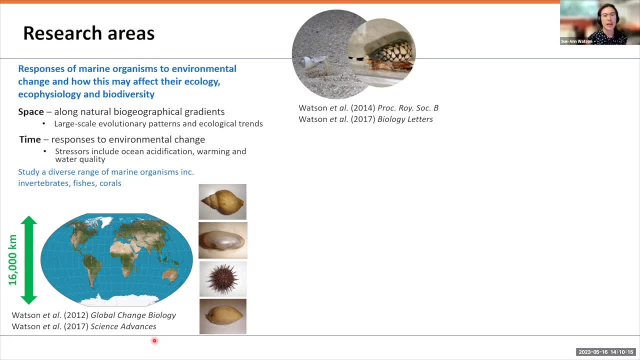 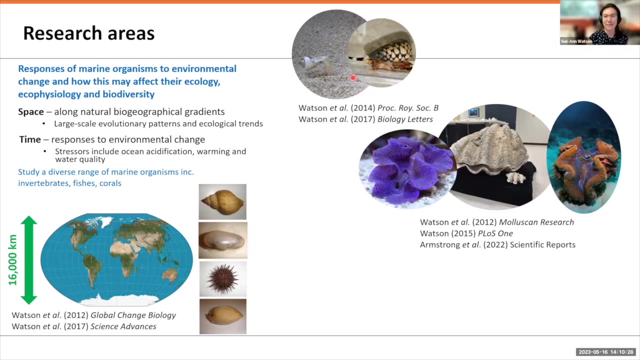 light warming and ocean acidification, and so here there's just a couple of examples, and we've actually been looking at how ocean acidification condition can alter behaviour. We also work with threatened species, so the giant clam example here, and you will hear more about that obviously in this talk- and that museum role really involves the collection. 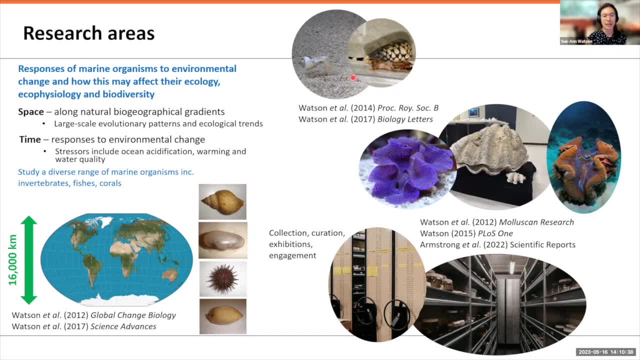 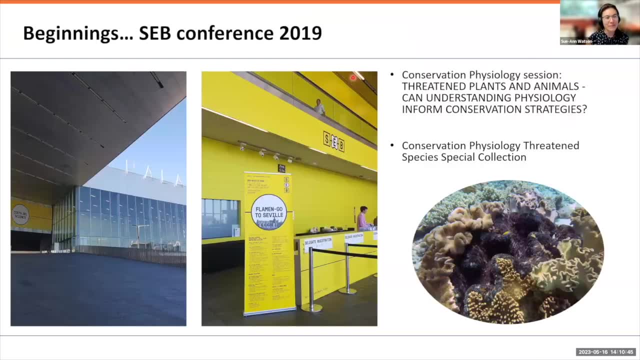 of new specimens, their curation, involvement in the planning of exhibitions and then engagement as well. So now to the story of the paper. so this paper really began in 2019 at the FCB conference that we went to, and so the paper, or the talk, was presented in the Threatened Plants and 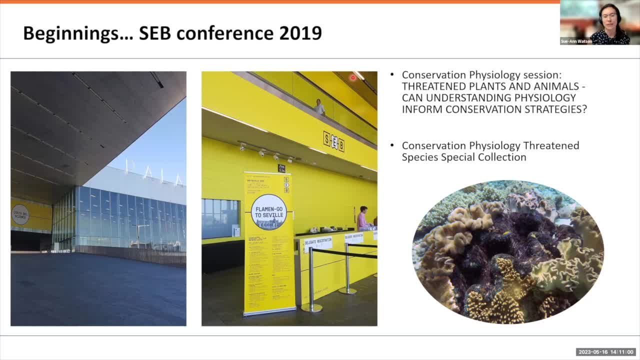 Animals session. Can Understanding Physiology Inform Conservation Strategies? As part of that session, there was going to be a special issue in conservation physiology on threatened species, And so I had the opportunity to talk about that. I had the last talk at the very last day of this conference and I had- yeah, I remember. 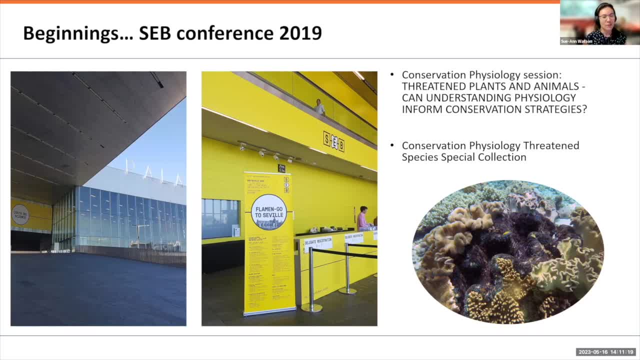 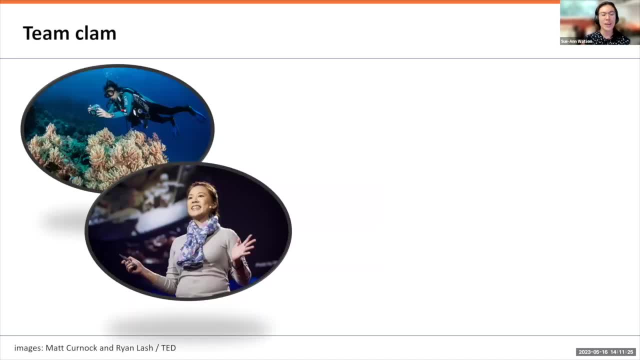 afterwards. we just had a chat about it, And so I thought that, yeah, I would write this paper, but I would need to sort of bring on a collaborator So who was going to be team clam for the paper, And so I decided that it would be really great to invite Mayling Neo onto this paper. 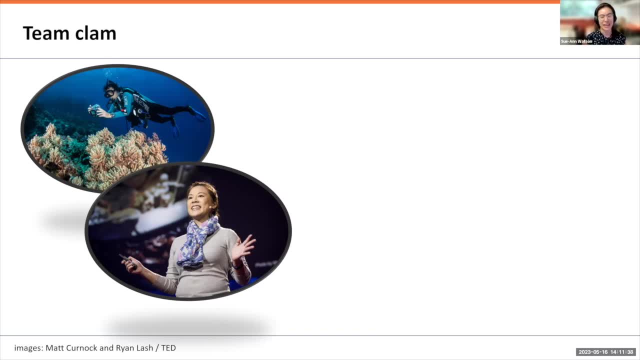 I've wanted to work with Mayling for a while. She is a giant clam expert And she has this really great background on working across all different species of giant clams, And I have more of that experimental and global change background, So I thought it would be really good. 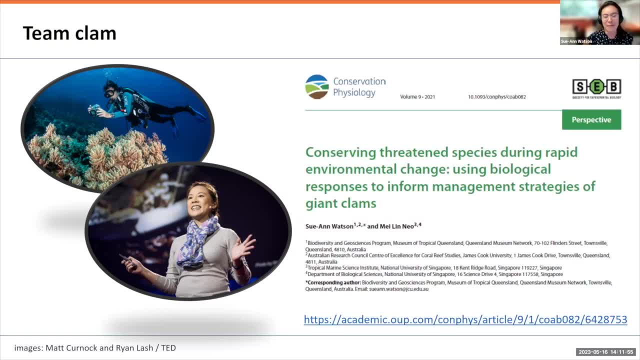 So together, in 2021,, we sat down and we wrote this paper. It was obviously virtual because no one was allowed to travel. Mayling is based in Singapore and I'm from based in Australia, And so we put this paper together. 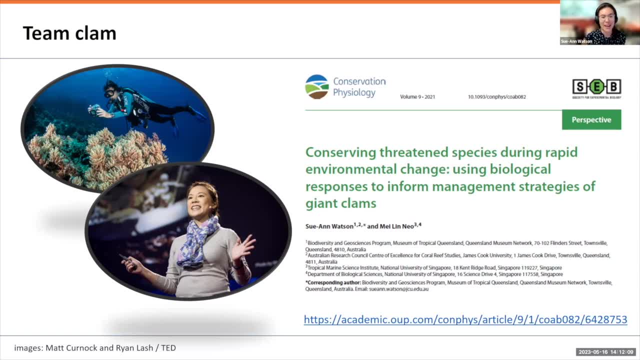 I think in about six months, Six weeks at the start of 2021, just using sort of the cloud. So we would just write paper when we were at the text, when we were in our different time zones, and then get on together. 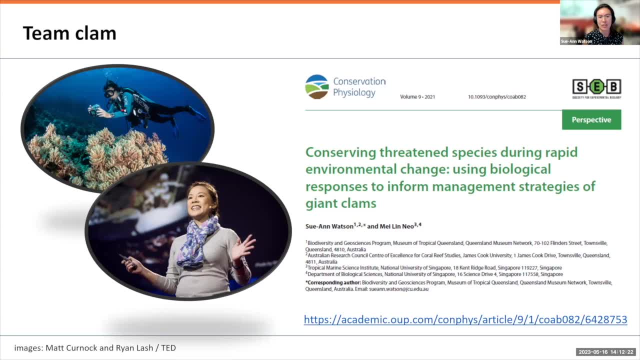 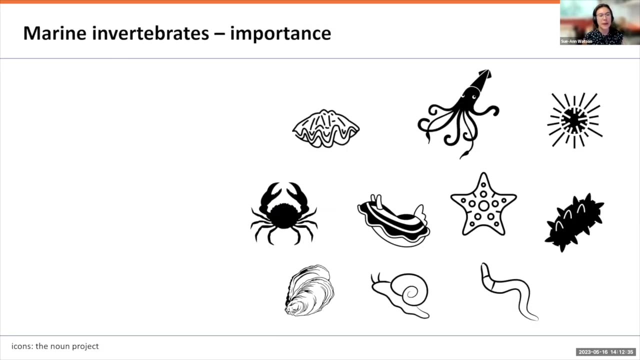 So it was a really fun collaboration to do. I really enjoyed the ability to sort of, I guess, be a little bit more opinionated in a perspective article than we might be in a normal sort of research paper. So the basis of why we did it. 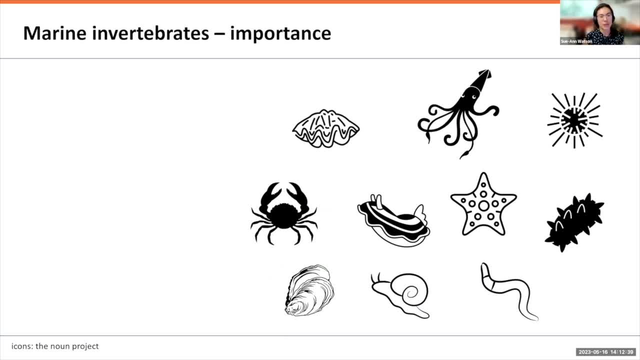 This is why we really wanted to study our marine invertebrates, and particularly giant clams. Well, invertebrates we find are so important. they're so biodiverse and they make up about 98, 99% of the animal diversity in the oceans. 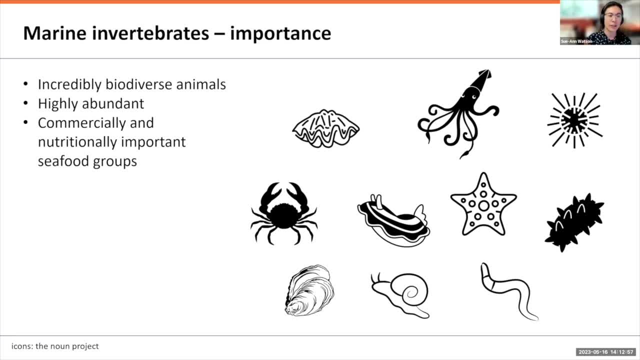 And they can be highly abundant and they can include commercially important groups. Cultural significance is obviously also important. They tend to really sort of form these fundamental lower levels in food webs which then structure marine ecosystems and traffic dynamics. And, importantly, invertebrates are actually often understudied on coral reefs, where people 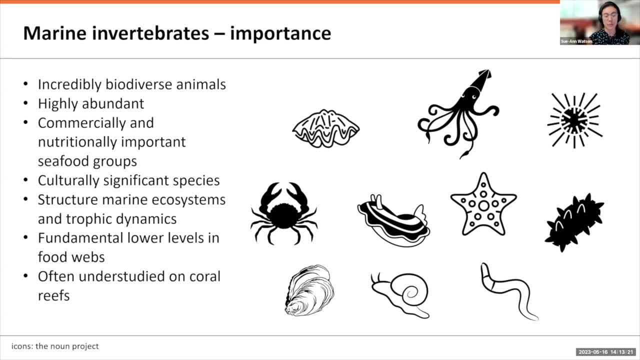 tend to work on the fishes and the corals, corals obviously being invertebrates, but you know ones that are quite sort of obvious and dominant. but there are this whole suite of other invertebrate species that often go understudied. 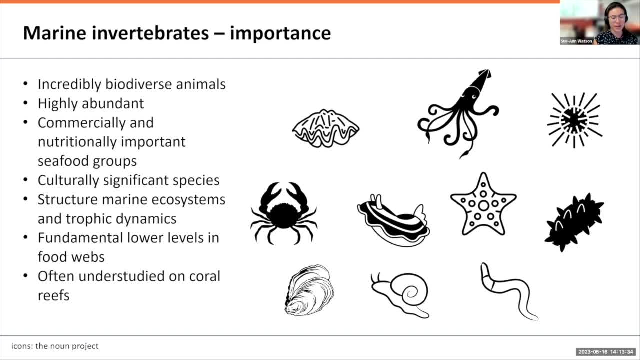 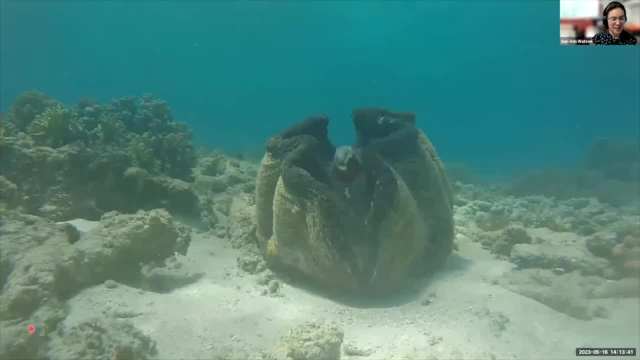 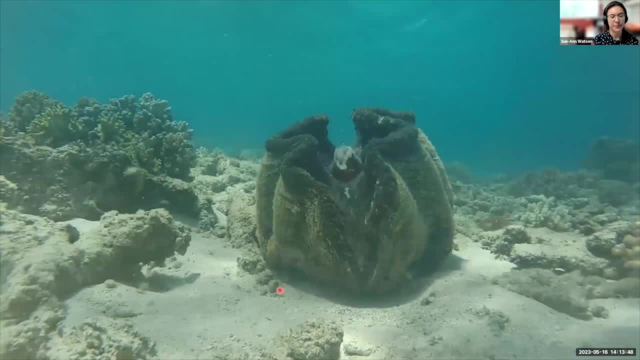 And so what we did is we looked at a number of invertebrates. We looked at a number of invertebrates, So one of those that we have chosen to work on obviously are the giant clams. So I thought I'd show you a bit about the giant clams, see if we can get this to work. 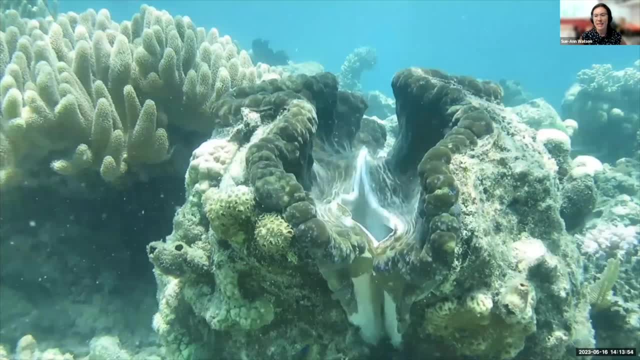 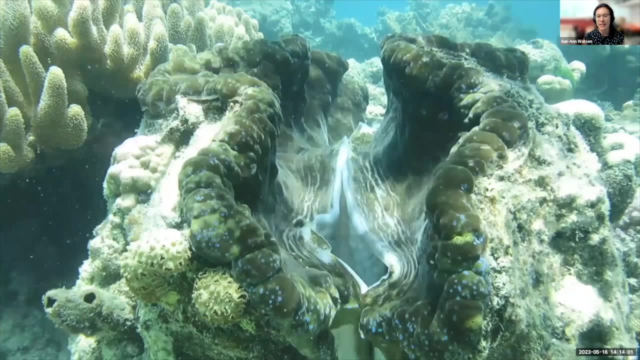 The giant clams. a true giant clam can get to 1.3 meters in length. They can weigh 250 kilograms and be around about 100 years of age. We project like trees that actually have rings in their shells, so you can actually count. 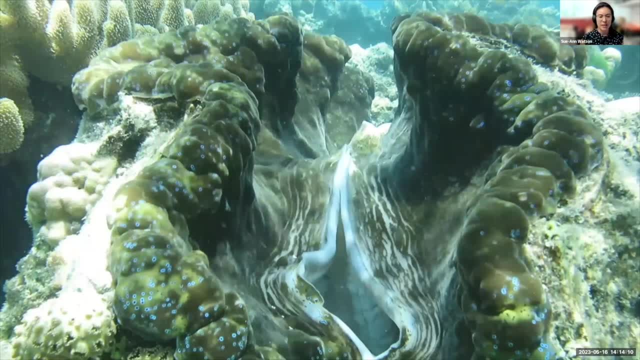 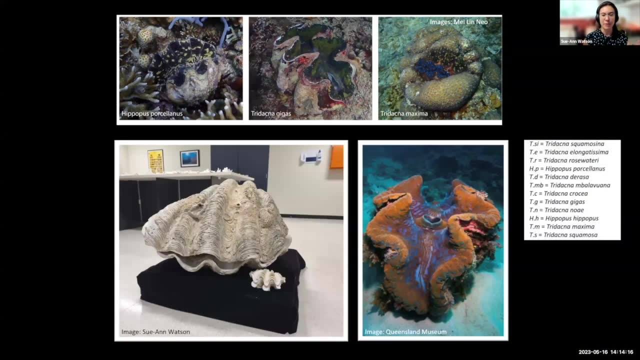 and age them. So importantly, once settled on to coral reefs, giant clams don't move. Here we have some examples of the 12 species of giant clams and they sort of really range in size, but you can see that they are large animals. 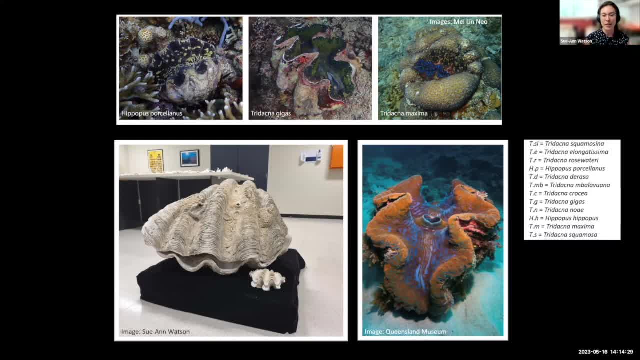 They have this planktonic larval phase and then they choose where to settle And that's it. they can't move. They also take a long time to reach maturity, So this could be sort of about two to 10 years. 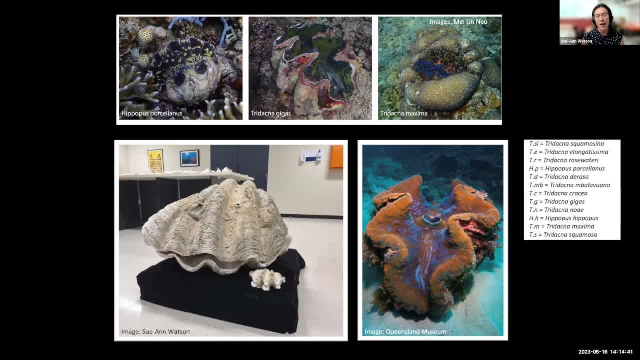 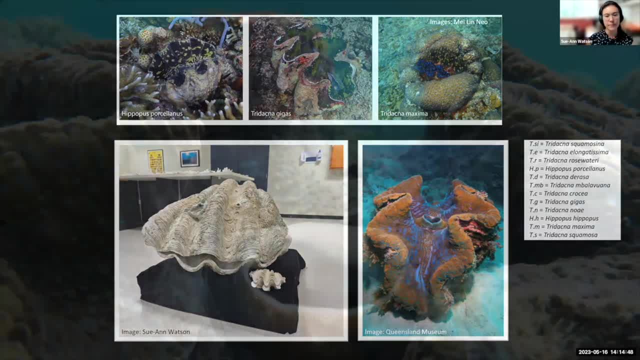 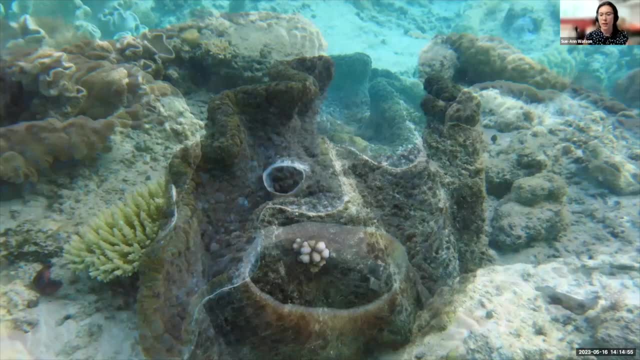 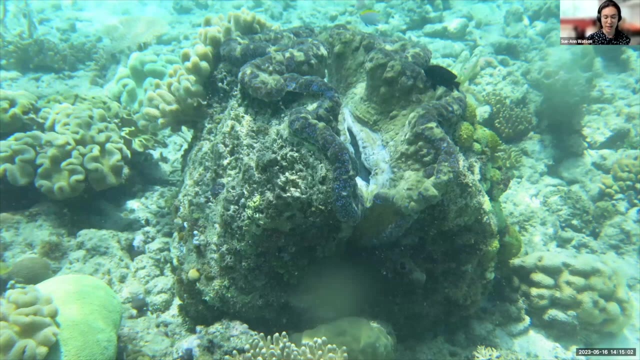 They start off as male, then they turn female And so they take that long time to really be able to produce those female gametes. So they can also have other important roles on coral reefs. So, for example, they Provide habitat for other, you know, for fish and coral and other animals. 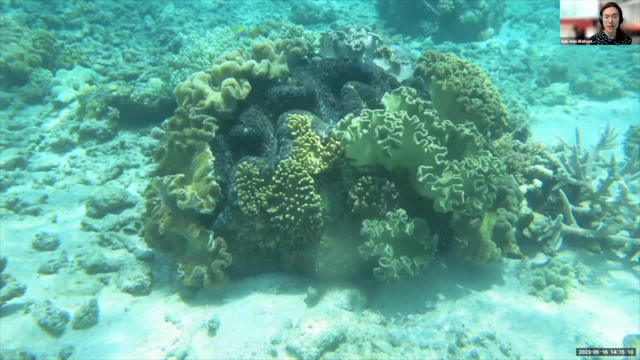 They filter the reef, so they're like the vacuum cleaners of the coral reef. They biofilter the food out of the water column And they're also important contributors to the carbonate budget. So, for calcification, they can provide up to 9% of the carbonate budget in areas like 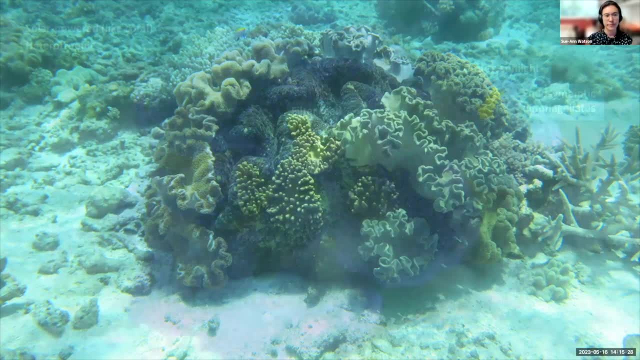 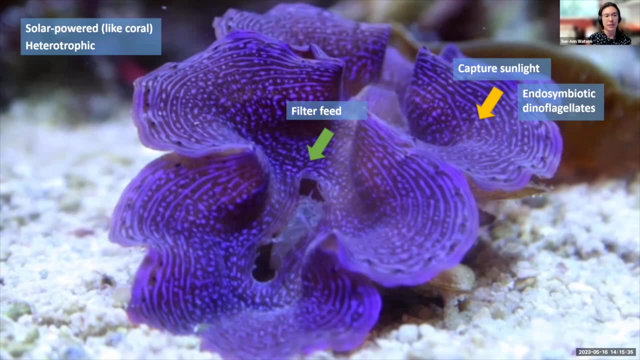 the Red Sea. Okay, Giant clams, as I mentioned, are actually solar powered and what this means is sort of the heterotrophic, So they can obtain energy by filter feeding and also through their algae and their tissues, which can capture sunlight and provide energy to the clam host in the form of sugars. 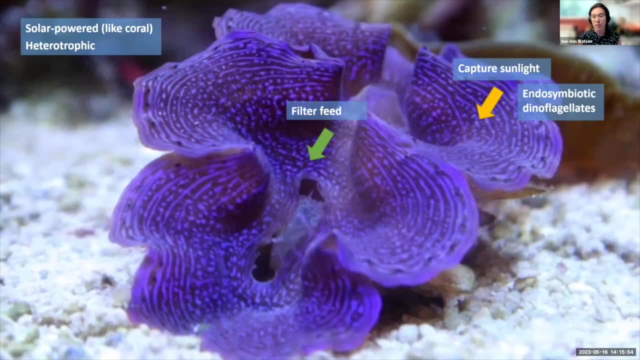 And this extra energy is one of the reasons that giant clams can really grow so big. So this is really good. They've got this extra superpower, But actually their superpower can also turn out to be problematic because, just like corals, 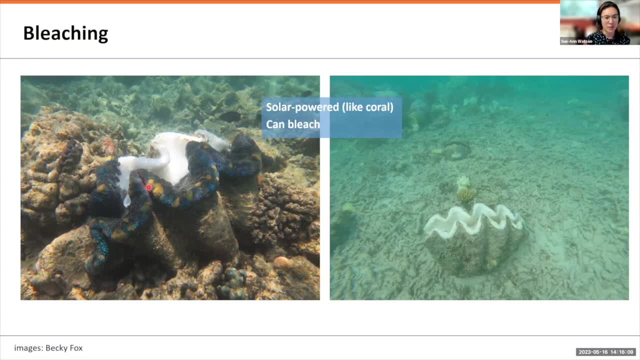 giant clams can bleach, And so this is a photo of a partially beached giant clam, and this is a completely bleached giant clam. This is a really large individual, And this photo was taken in 2016, during the 2015-16 coral bleaching event on the Northern. 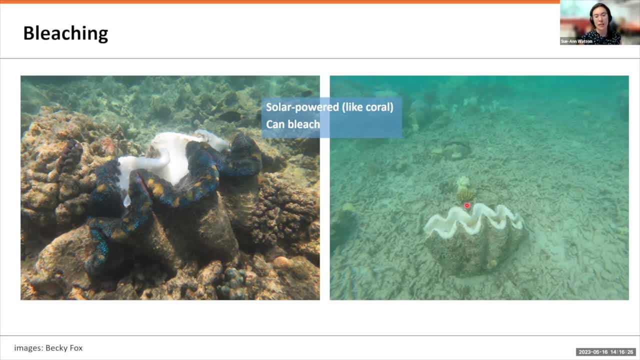 Great Barrier Reef And this individual later died. So what happens is that the giant clam expels all the symbiotic algae from its tissues. The tissues are white, but then it doesn't get enough energy, And if conditions stay like that for too long, then it will die. 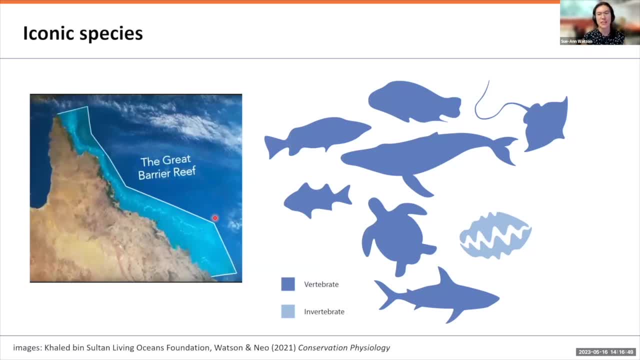 The giant clams on the Great Barrier Reef are actually considered iconic species. Of the eight key iconic species to see, The giant clam is the only invertebrate, So I guess they were quite interesting in that sense. They're actually also the only one of those iconic species that stay set in their same. 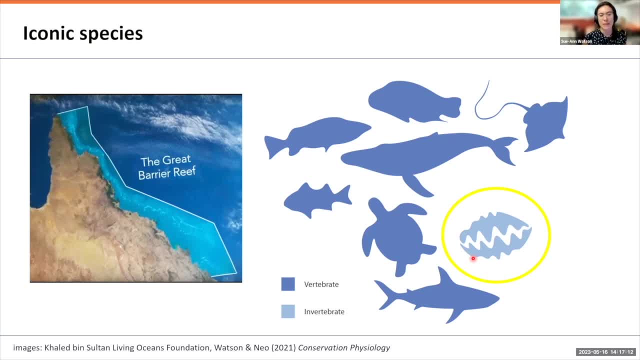 location, which means that tourists going out to see them are guaranteed a sighting, whereas those other organisms can move around a bit more. Now, the giant clam is a very big species And it's very, very large And it's very, very small. 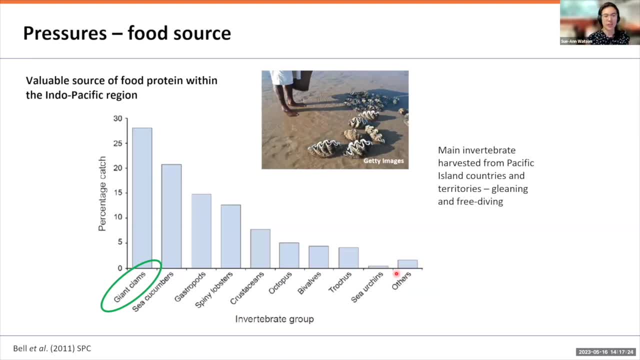 And it's very, very big, So we can kind of see how large it is And the giant clams are faced with a range of pressures from humans. They're a valuable source of food protein within the Indo-Pacific region And actually the main invertebrate harvested from Pacific Island countries by gleaning. 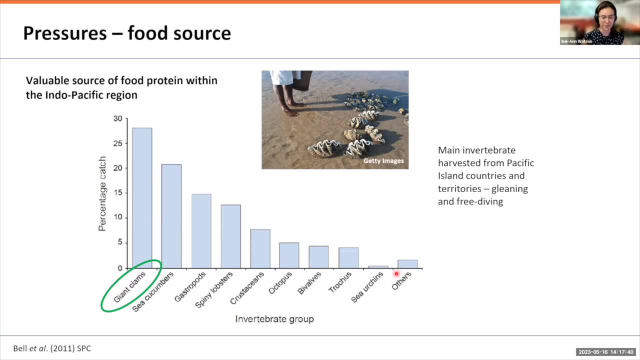 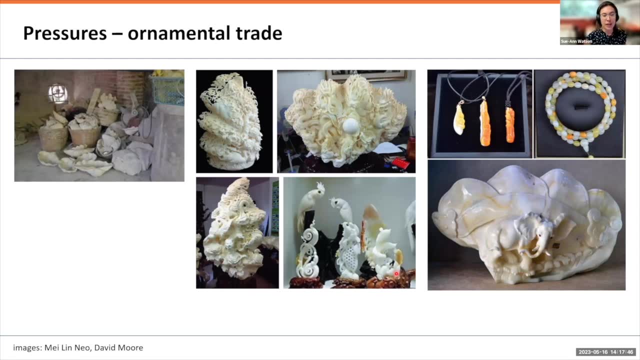 and freediving, So they face a lot of pressure there. Giant clams also face pressures from the ornamental trade, So their shells are used to make these beautiful carvings- beautiful carvings, and also they're recently sort of a key animal traded in the ornamental 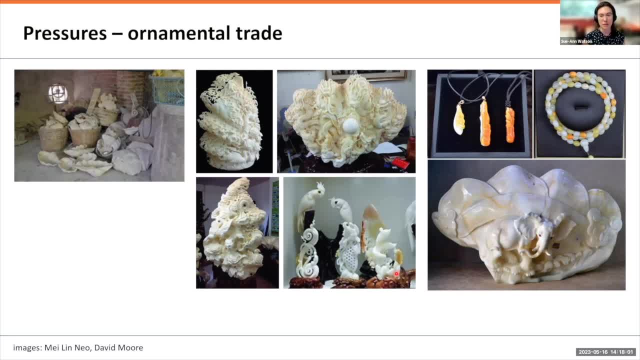 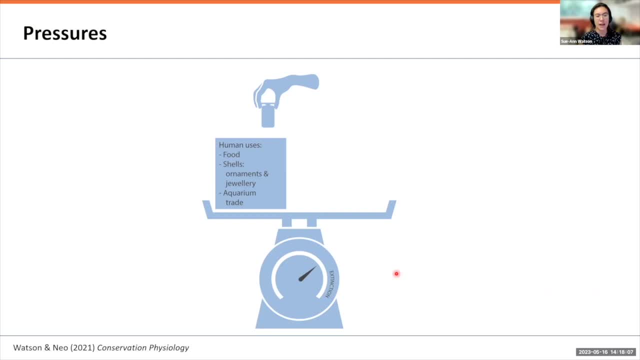 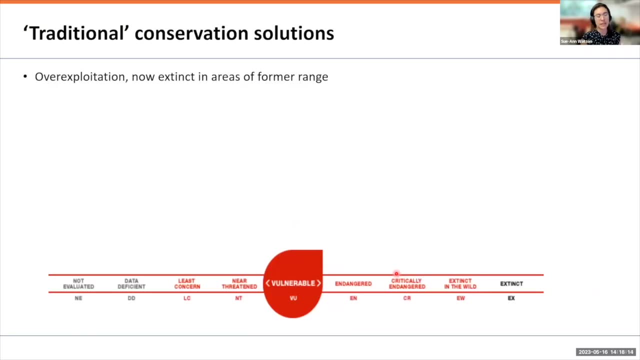 aquarium trade as well, so people will keep them in their tanks as reef pets. So there's a range of pressures that giant clowns face and that is sort of, you know, pushing them potentially to extinction. Now what we're seeing is that, because of over exploitation, giant clowns 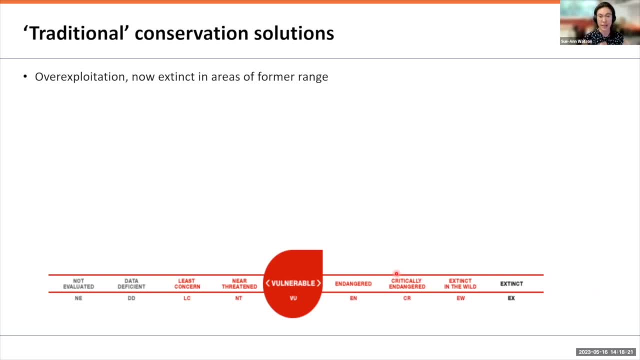 are now extinct in areas of their former range. they're actually sort of retracting in their range and so traditional conservation solutions to try to help with this and include giant clowns being societies, listed species, so actually protected under appendix 2, and international trade is banned. 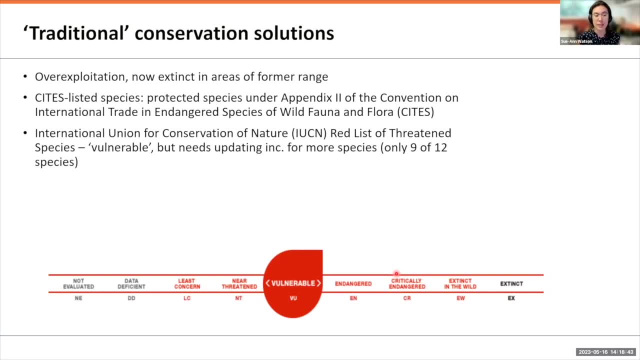 Giant clowns are also on the IUCN red list of threatened species. They're listed as vulnerable for several species, but this currently needs updating because only nine of the 12 species have been assessed. Conservation efforts that have been underway to address these problems of over exploitation. 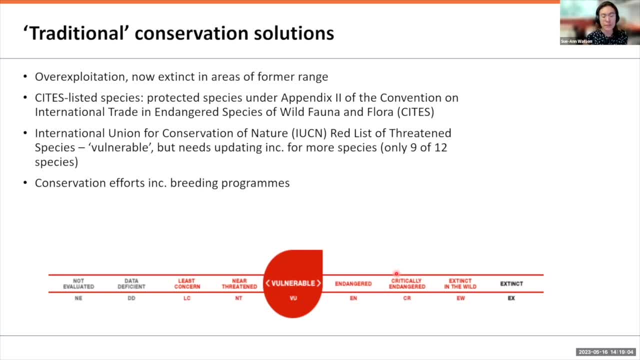 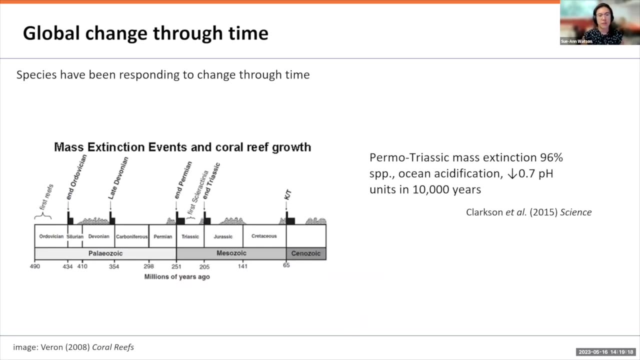 include breeding programs, and these have been quite successful in local areas. However, there are new challenges that we're realizing giant clowns are facing, So we know species have been responding to change through time. On coral reefs, for example, we've had five mass extinction events in the past. 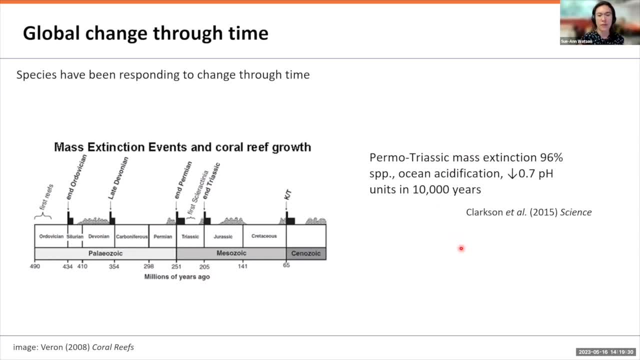 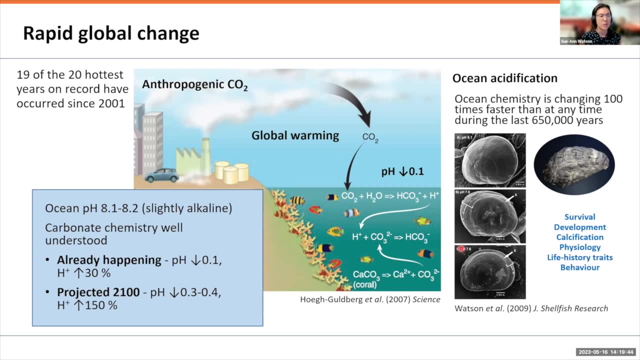 and we can get ideas of the kinds of rates of global change, including ocean acidification in previous mass extinction events. But what we're seeing now is this really rapid global change? For example, 19 of the 20 hottest years on record have occurred since 2001.. 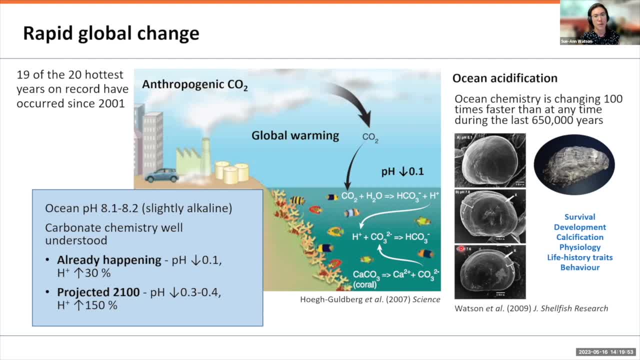 Oceans take up 90% of the heat that we emit from burning fossil fuels, and they also take up about 30% of the carbon dioxide. Once in the oceans, the carbon dioxide reacts with water to form carbonic acid, And there's this acid that causes ocean acidification. 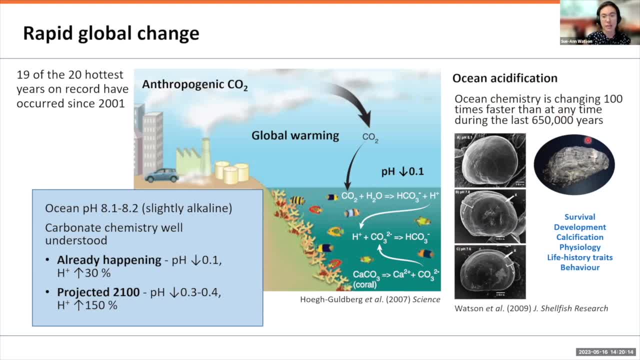 We know ocean acidity chemistry is changing really rapidly and actually potentially more rapidly than several million years. Ocean acidification causes problems for animals that make calcium carbonate, all these limestone shells and skeletons. It includes problems with their survival, development, calcification, physiology, other genes that don't rely on carbon. le tow rage or local ion molecular�� stopping a disease in the body, or Metropolitan Institute of Science and Science did a trial last year In Australia. these plants are companiishes of Aries Never Voor, 24 year old, produced carbon dioxide acid. There's another January 그. 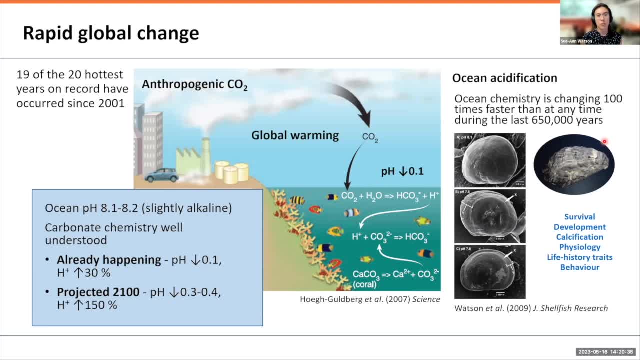 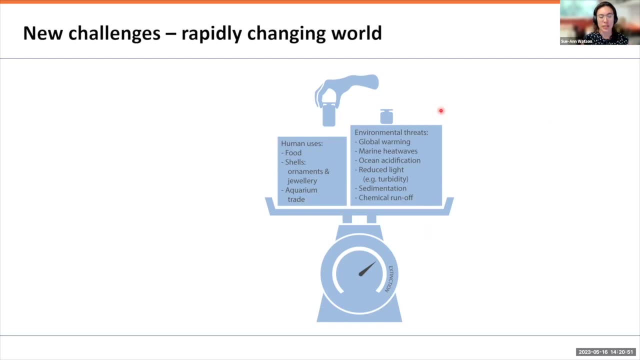 general life history traits, and also we're finding problems in behavior for animals that even don't make a calcium carbonate shell or skeleton like squid. So our giant clams are facing these new challenges in a rapidly changing world. They include some of those global scale drivers that I mentioned, and also some additional ones that we considered in. 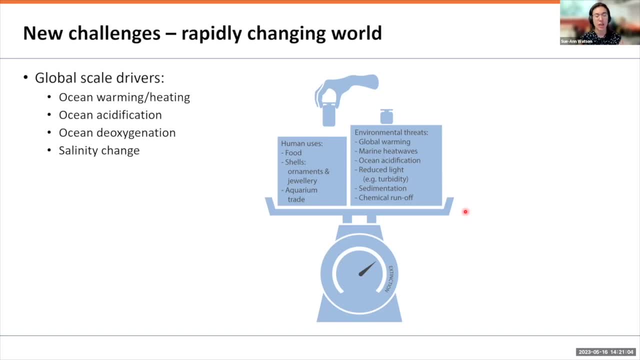 the paper, including deoxygenation and salinity change As well. giant clams face local to regional scale drivers that could cause stress, including light availability, which may be altered by processes of agriculture and urbanization that lead to turbidity and sedimentation in the water. 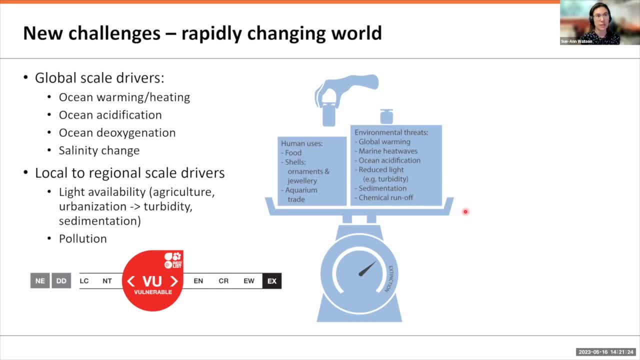 Giant clams also face pollution, which might be physical in terms of, say, plastic material or more chemical. So we really started some of this research with asking the question: how can experimental findings inform the management of giant clams and indeed other solar-powered organisms, potentially such as? 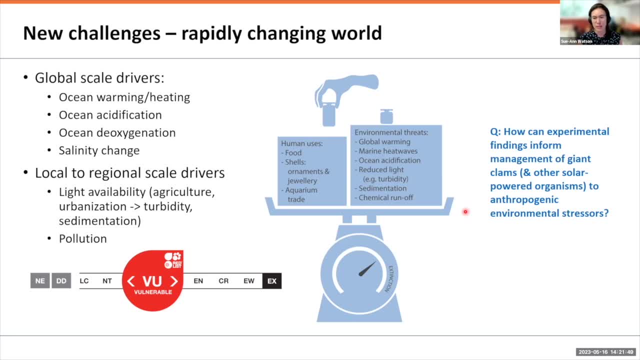 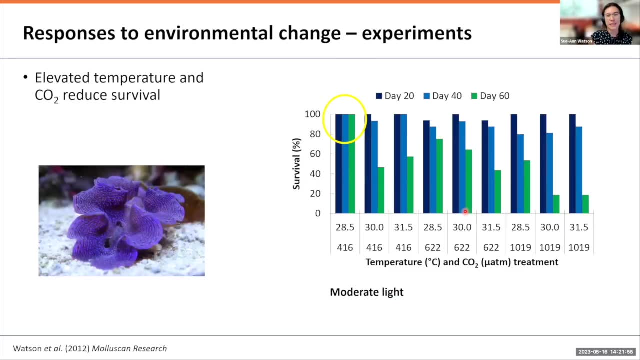 corals to anthropogenic environmental stresses. So we run some experiments and these are sort of this is based on some other experiments that we've done. So we've run some experiments and these are sort of this is based on some other papers that we have made and we really started to find out at this point that elevated temperature. 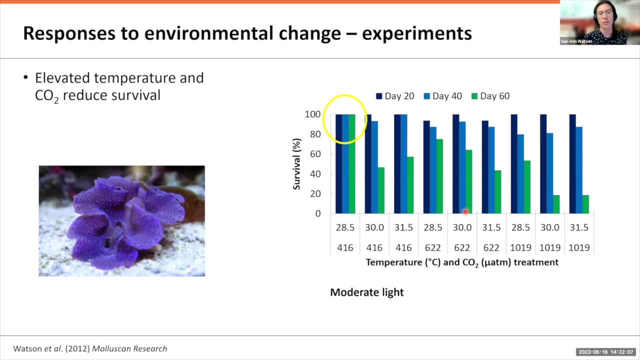 and elevated carbon dioxide levels tend to reduce survival in giant clams. So here this is after 60 days, and you can see that the increasing temperature here leads to a decrease in survival, whereas increasing temperature and increasing CO2 leads to sort of the most dramatic decreases in survival. 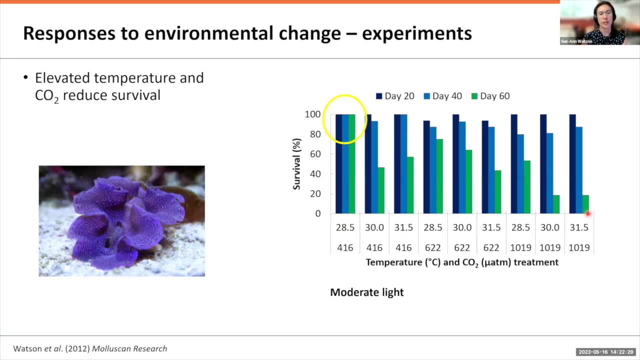 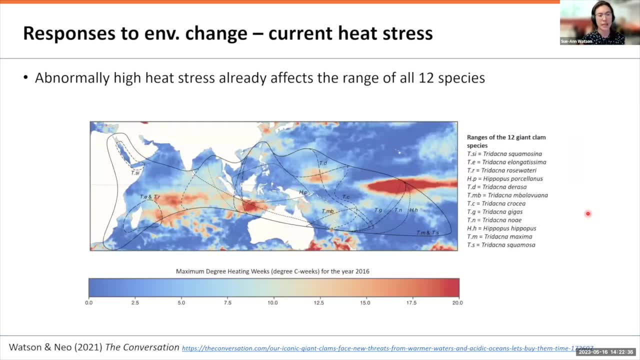 And so what we started to do is we started to look at what we could do with giant clams, and what we wanted to do was to sort of build on those findings from that research and say, okay, so what's happening currently? Well, actually, what we can see is that abnormally high heat stress already affects the range of all of our 12 species of giant clam. 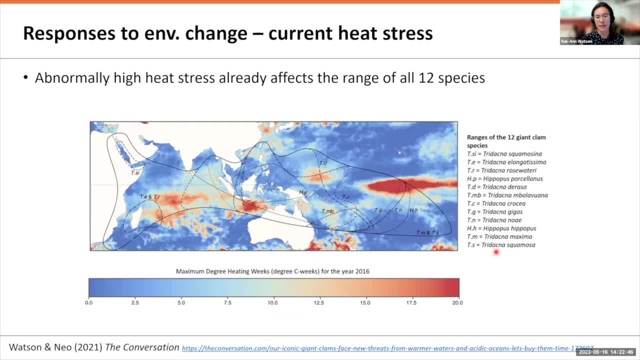 That's our 12 current recognized species, and their abbreviations and names are listed here, And so this is really interesting, because that Indo-Pacific warm pool and wet temperatures are permanently over 28 degrees- has expanded nearly two-fold in the last 40 years and now covers much. 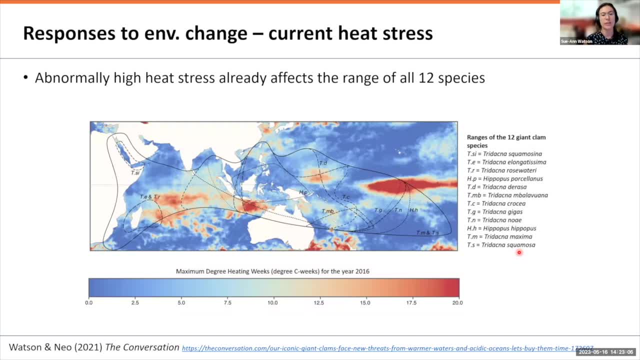 of the Indo-Pacific region. So we're seeing this overlay of heat stress, plus in certain years- and this is for the year 2016- you can see that sort of the red colors and the sort of the orange colors being heat stress that we don't normally see and but that's really present in in large areas of the range. 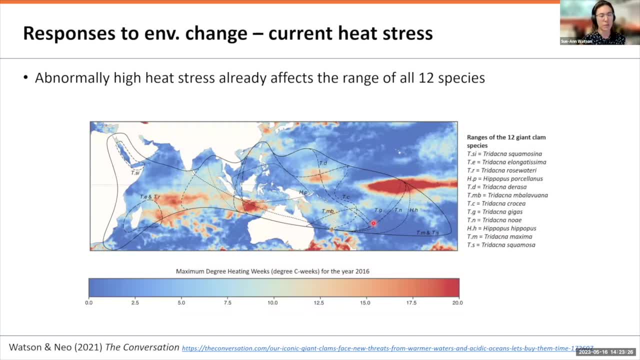 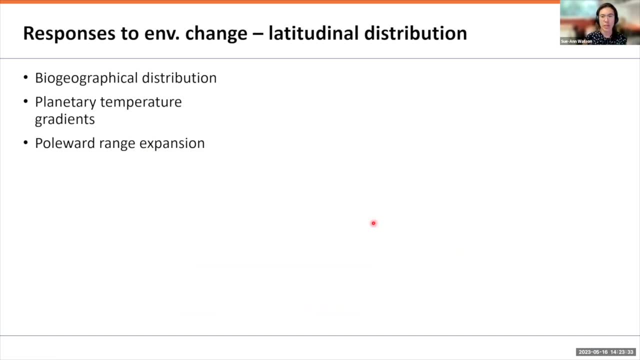 So it's not really a future problem, it's a current day problem for heat stress. Now animals can respond to heat stress by changing their latitudinal distribution, so, for example, they can move south in the southern hemisphere or north in the northern hemisphere and take advantage of. 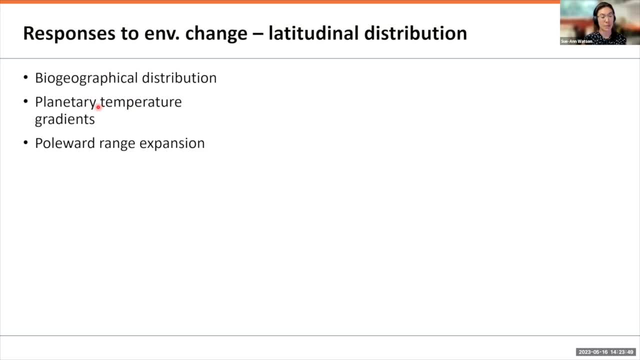 the planetary temperature gradients and it should exhibit a poleward range expansion. And actually there are millions of other species in the southern hemisphere that do this more than just heat stress, But I'm pretty sure that they're orthodontic and we can see that almost all of them are using heat stress. But if we looked at all these animals in this particular form, it would seem that they have no direct displays of heat stress. and we took a look at them and we said, well, we've got one that's a little thinner, one that's lighter, and the other is earlier than the other. 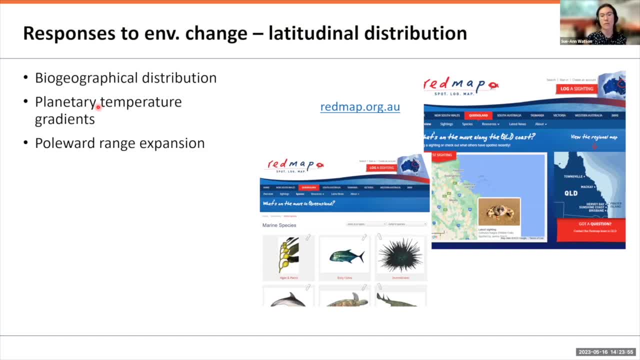 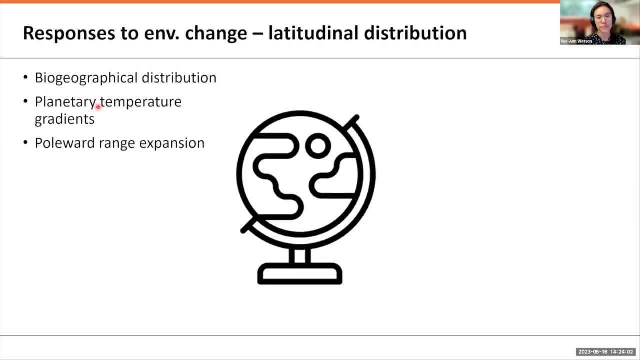 are citizen science projects that measure this. i'm involved in one called red map here, where we're tracking species moving along coast around australia. so for giant clowns, herba- the problem with the pole range expansion is that as you move towards the poles, temperature does decrease, but also you get saturation state decreasing. now this is the 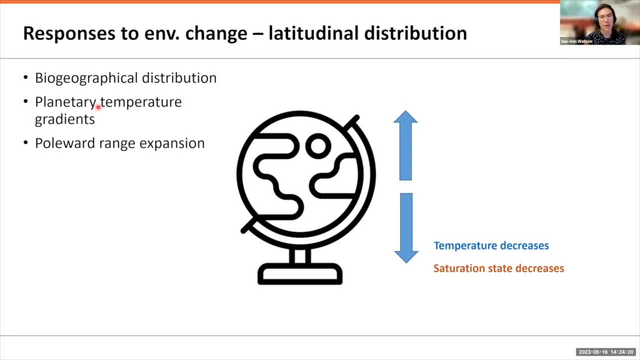 measure of the saturation state of sea water with respect to calcium carbonate polymorph, which is what giant clams used to make their shell. aragonite is the major polymorph that giant plants will use in their calcium carbonate shells, and aragonite saturation state decreases as you. 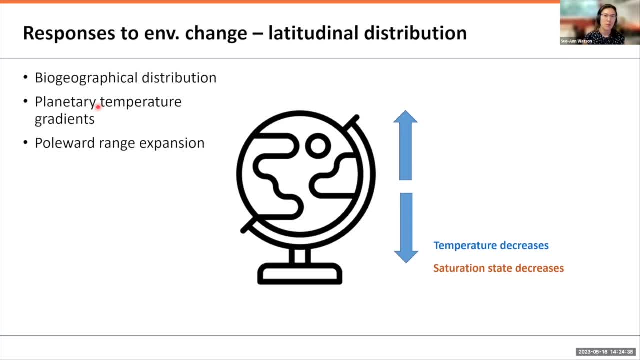 move the water towards the poles, which means it's more difficult for giant clams to make their shells as they move towards the pulse. what we also see as we make pole woods is that these light levels decrease. so it seems like for giant clams, moving pole woods isn't going to be a very viable option, and instead, what we're going. 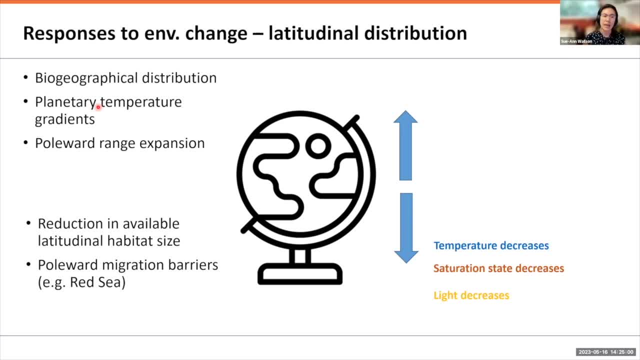 to see is temperatures. warm is a reduction in available latitudinal habitat size. additionally, in certain areas for giant farms we even get a pole with migration barrier, such as in the red sea. so giant clams wouldn't be able to move any further north because of the. 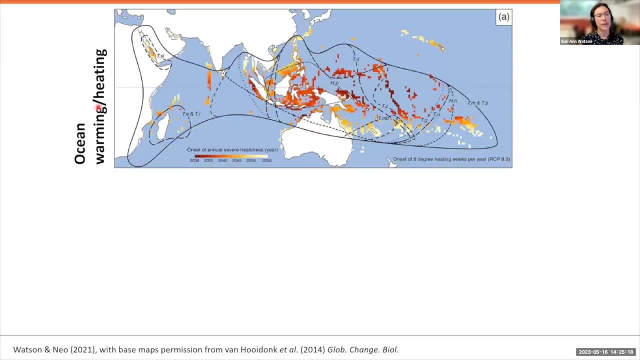 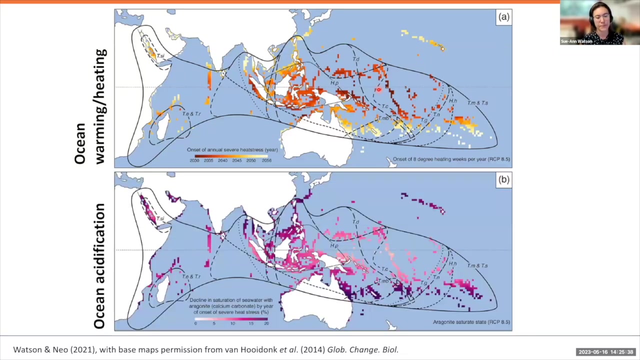 higher the red sea ends. so what we tried to do here was in a couple of maps in the paper we had a look at the effects of ocean warming and heating. and so here the: the onset of severe heat stress occurs most rapidly in the most equatorial areas, in giant clam ranges, and the onset of the worst um stress. 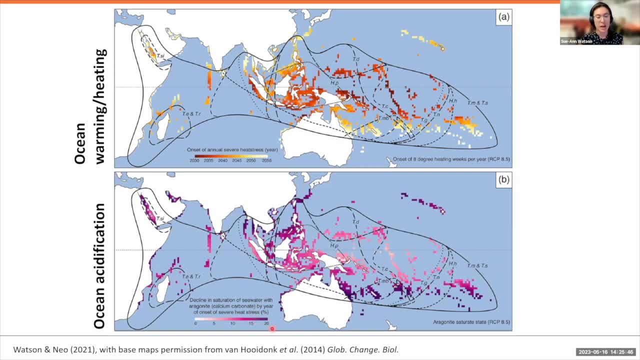 in terms of ocean acidification. so the greatest decline in aragonite saturation state occurs um closer to the poles. so what you can see from this diagram is that there's essentially no safe haven here for giant clams. they're either sort of hot or it's hard for them to make their. 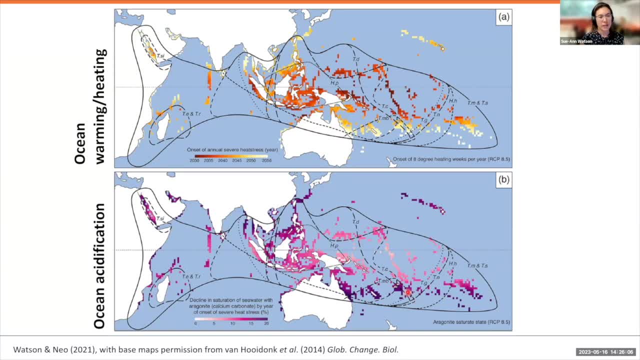 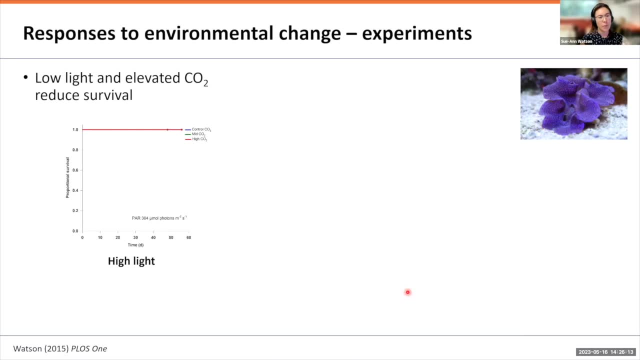 shells, the kinds of other factors that we included um in terms of our unknown experimental response is, and well, what we know about how giant clams perform at low light and high co2. so, if we look at three levels of carbon dioxide conditions in high light, the survivor of giant 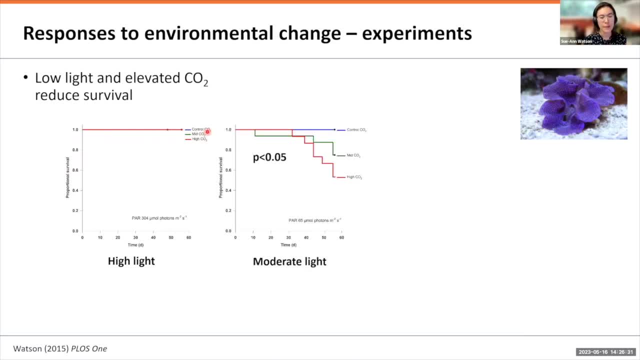 farms after 60 days stayed the same. however, as we decrease light levels, we can see that we were getting reductions in survival at these mid and high co2 levels, but not in the. then, if we went to very low light levels in our experiments, we got reductions in survival at. 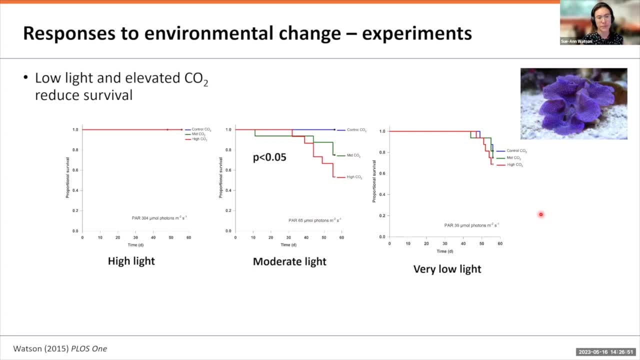 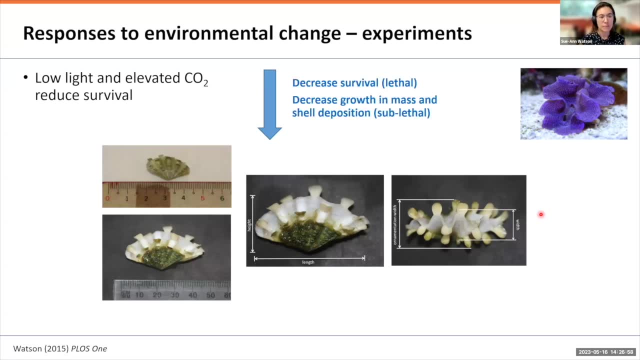 control mid and high co2 levels. we also know from my experiments that what we get at low light and elevated co2 is a decrease in survival, as i mentioned, which is a lethal effect, but we also get a decrease in growth in terms of mass and shell deposition. so these are some of the 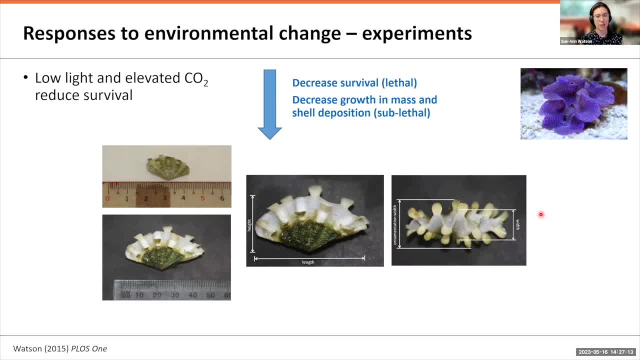 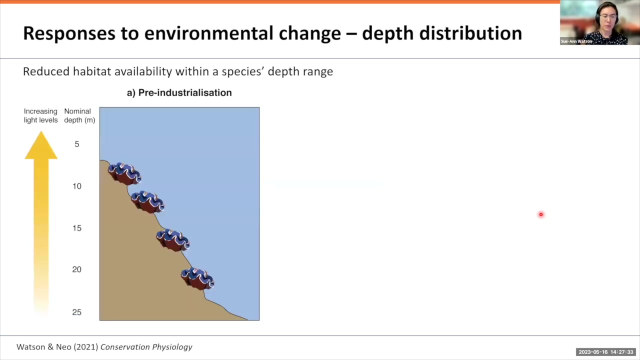 lethal effects that low light and high co2 are causing in our giant camps, and we know this from doing sort of our eco physiology type experiments. so what we wanted to do with this information is to project how these threatened giant clowns might respond on the reef in the wild. so if we had so we 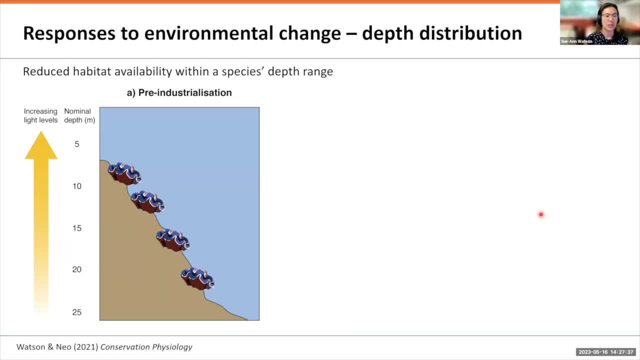 drew a conceptual model. so pre-industrialization, this is the, the depth range of giant fans or reef for many on the reef for many species. and then we thought about: okay, so what's happening in the present day? well, in the present day, what we have is this pressure on the upper depth range. 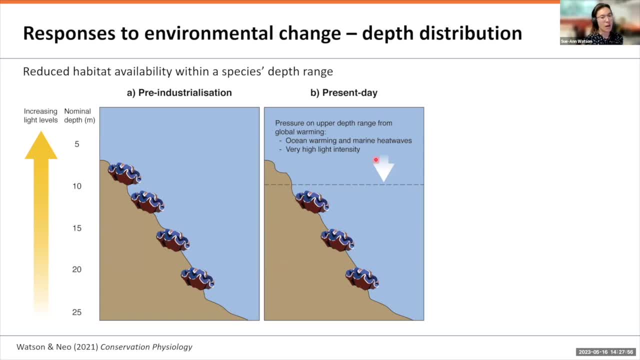 from ocean warming, marine heat waves and very high light intensity. so, as you can see from those bleaching photos, and we're tending to lose those individuals, and particularly those ones that live in the very shallow waters. and then we continued so, in future oceans, what we know from 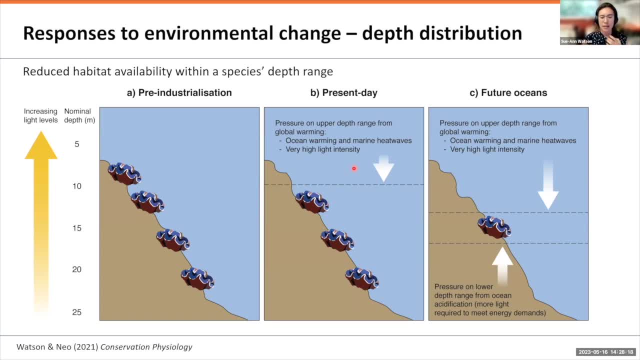 those experiments that i just talked about is that there's likely to be pressure on the lower depth range from ocean acidification. so the giant clams are going to need more light to meet their energy demands as oceans acidify into the future. plus, there's going to be continued pressure on 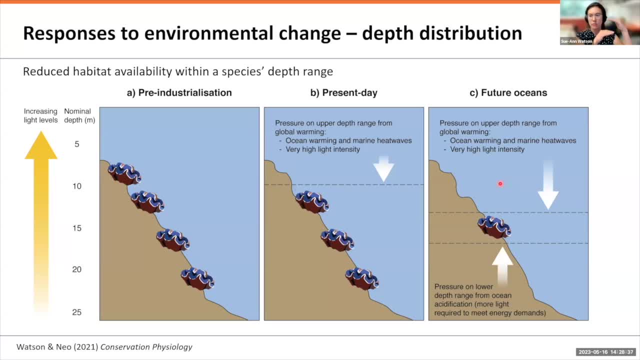 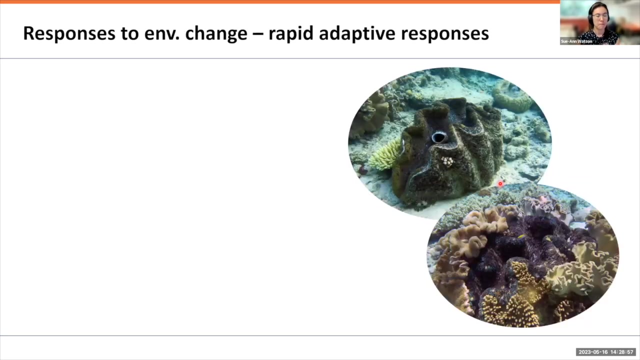 their upper depth range and overall this is likely to reduce the habitat availability within a giant clam species depth range. this approach is kind of conceptual model. what we think may well be applied to other sessile photosymbiotic animals such as reef building corals. so we also thought about 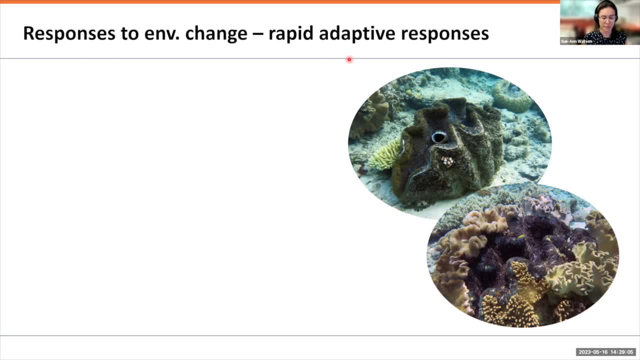 how we could reduce the habitat availability within a giant clam species depth range, how giant clams may be able to adapt and whether there were any kind of rapid adaptive responses that might occur. so actually, in giant clams they're able to open and close their shell somewhat. 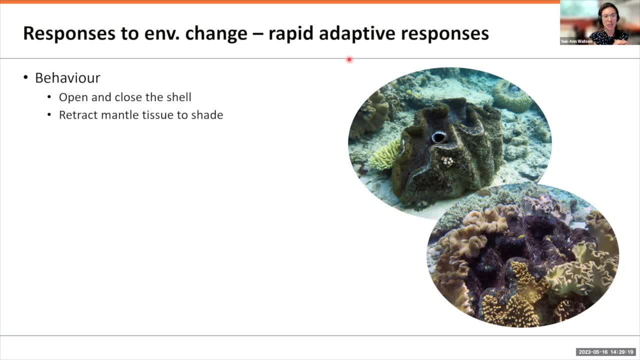 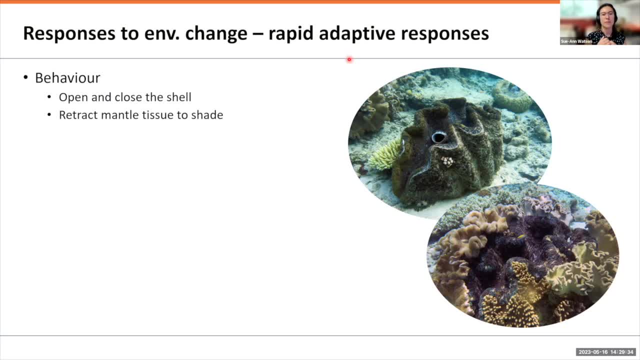 sorts of things that are producing stress. so this is related to the fact that Peacewaterhouse was released in 2013- it was an Phase IV of the Age of Manure- and Foundation study to not only tackle a better type of food- food but alsocile to fish predation, but also allows them the ability to escape some of the extra high sunlight and UV radiation during periods of stress. we also know that the giant clam is considered a hollow biome, so, as well as the animal, it has the plants, the algae, as well as bacteria, fungi and viruses associated with it. and so the giant clam as the hollow biome То adorable giant clam and all of thehabitants biomesauso the deeper order of plants and algae, as well as bacteria, fungi and viruses associated with it. 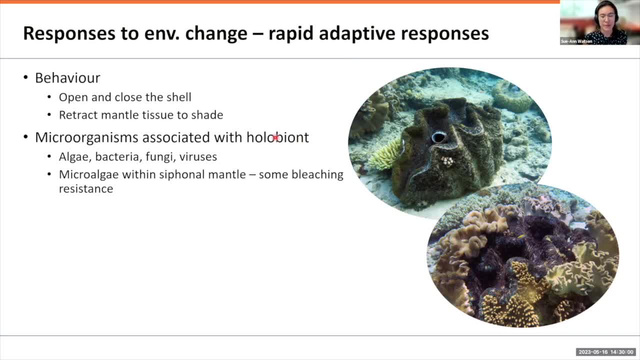 the whole, that was going to cause a очень great delay, especially as we began to move on to the next microaggression. And although giant clams themselves have this really long generation time, the microorganisms associated with giant clams have much shorter and more rapid generation times. 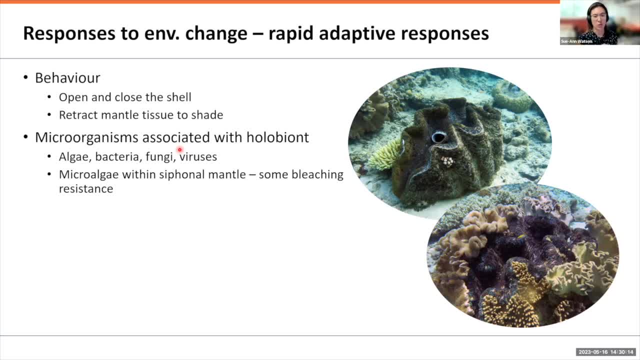 And so there is potential for these to display some genetic adaptation and so overall display a rapid adaptive response for the holobiont. In addition, the giant clam holds its microalgae within its mantle tissues, And this is actually different from how coral hold their symbiotic algae. 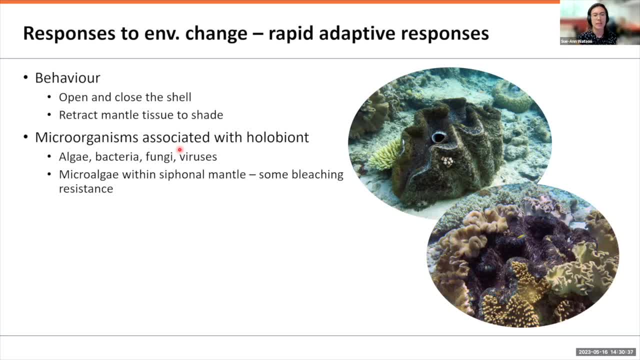 And so this could confer some bleaching resistance in the clams. Now we also know that organisms display phenotypic plasticity and, of course, the ability for genetic adaptation. However, because giant clams are long lived, and so giant clams that spawn in today's oceans are potentially going to be alive to the end of the century, and they'll only get developmental acclimation to today, 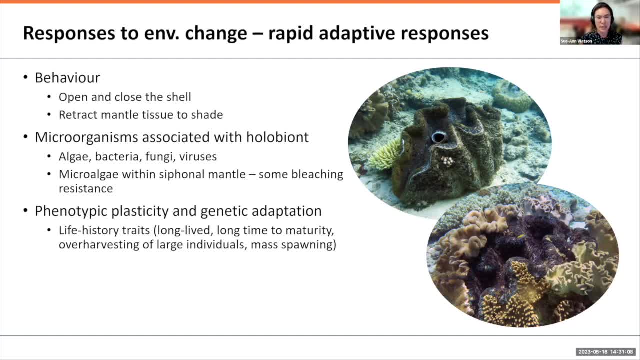 As well as that, they take a long time to reach maturity, so that generation times are more limited compared to other reef animals. And add in, the over harvesting of large individuals, which are the female ones, means that finitioning phenotypic plasticity and genetic adaptation may be a more limited response in giant clams. 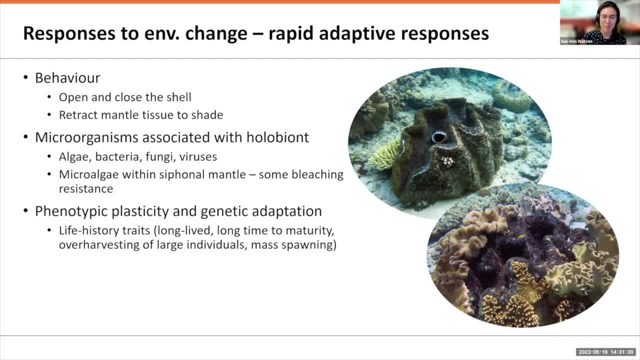 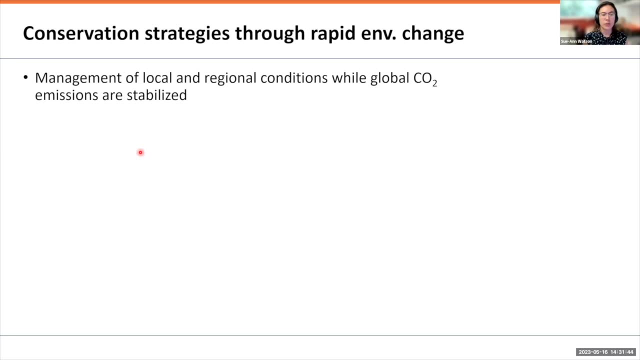 On the plus side, though, giant clams do have mass spawning events where millions of gametes are released into the water column, allowing a massive potential for selection. So what I wanted to talk about now is some conservation strategies that we could use through rapid environmental change. 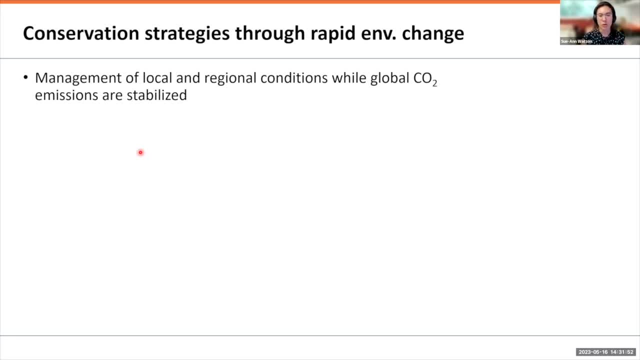 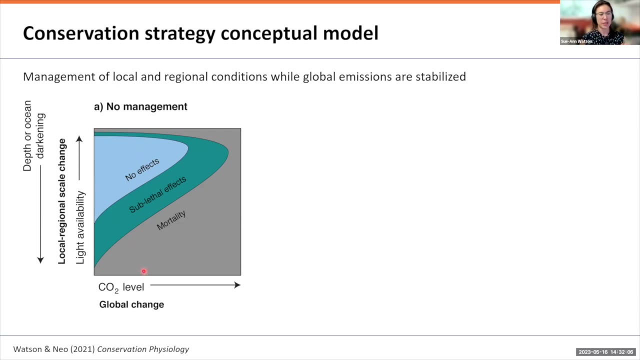 And I'll first talk about the management of local and regional conditions while global carbon dioxide emissions are stabilized. So for this we drew a conceptual model, And what we put together was, if you can imagine, the reef image that I showed you before, so giant clam depth distribution on the reef. 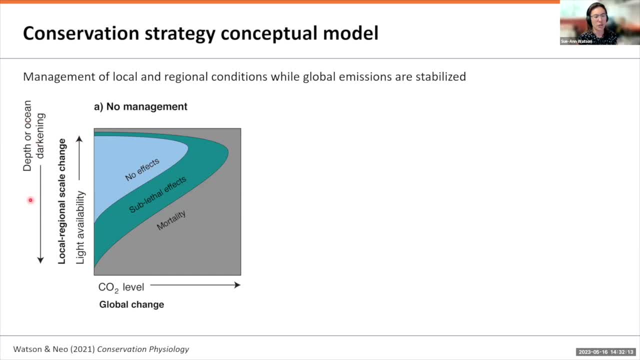 And so this is the same on the Y axis. so depth or ocean darkening that might be caused by turbidity or sedimentation And then light availability up here. So these tend to be local to regional scale, changes caused by the influence of activities within the catchment leading into the water. 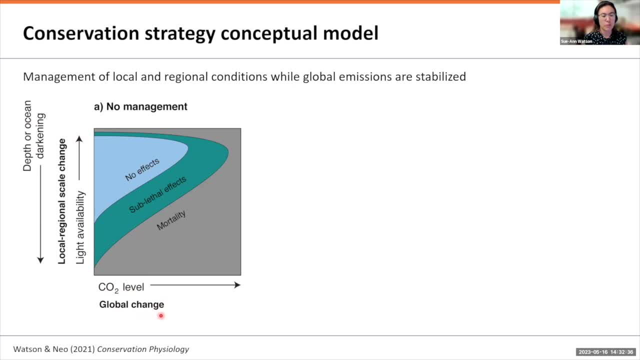 And then on the X axis we have sort of this global scale factors, mainly CO2 level, which leads to temperature, increased temperature and carbon dioxide, And so we can see we have this sort of sweet spot here of no effects. So this is where giant clams would like to live, on the reef. 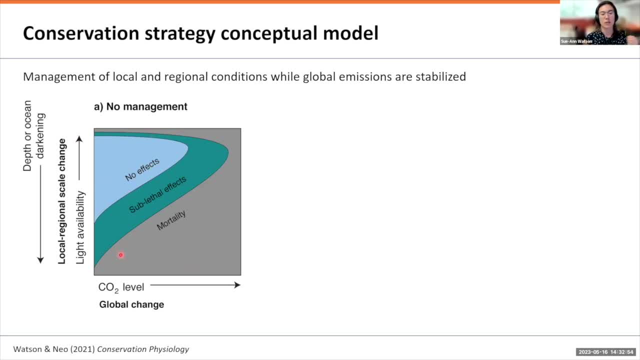 This is sort of too shallow for them and this is too deep. There's not enough light, And then within the range it's sort of out of the no effects range. we have sublethal effects and then we have mortality. Now what we thought about when we wrote this paper was that if we could improve water quality to enhance light levels on a local scale, then we would be able to do that. 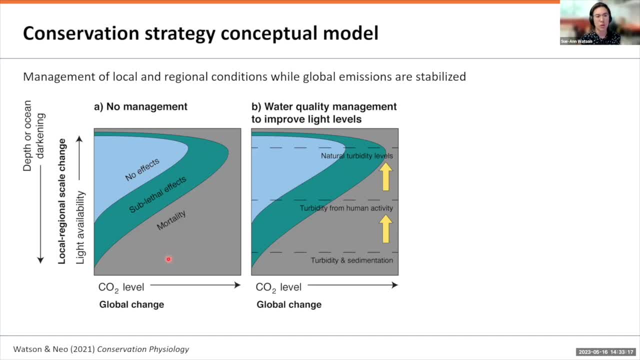 So if we could improve water quality to enhance light levels on a local scale, this might help to conserve giant clams by improving the water conditions while global emissions are stabilised. And so, if we think so, if we had turbidity and sedimentation, 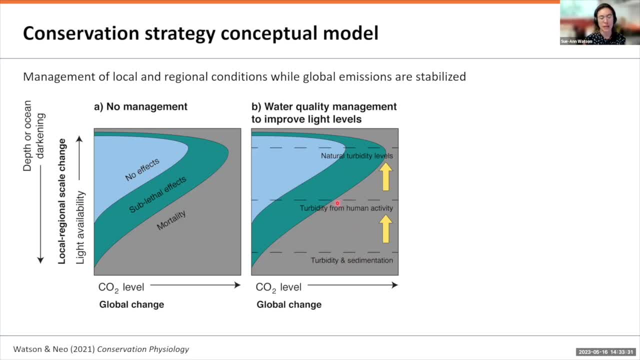 So if we perhaps remove some of that turbidity from human activity, we end up with better light levels in the water And then we do that again, We might start to move giant clams from these sort of sublethal effects and mortality levels. 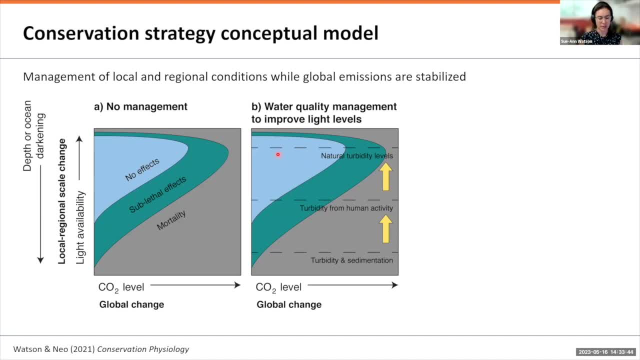 Up to the better area of no effects And then, of course, with carbon dioxide emission reductions, if we get to net zero by 2050, or if we get to net zero by 2035, this is going to have an effect on where we end up in terms of CO2 level. 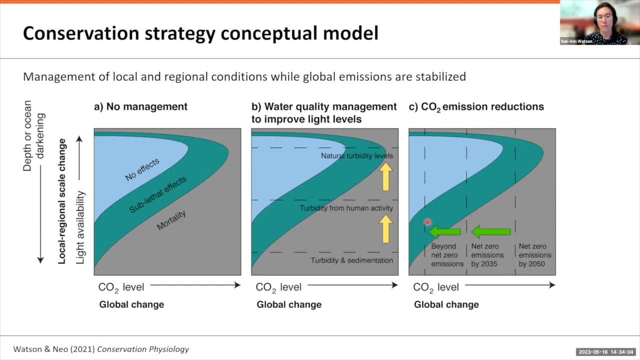 And then if we get to beyond net zero emissions and we get to push back, this will move that x-axis back. So this is a way that we sort of try to conceptualise. So this is a way that we sort of try to conceptualise. 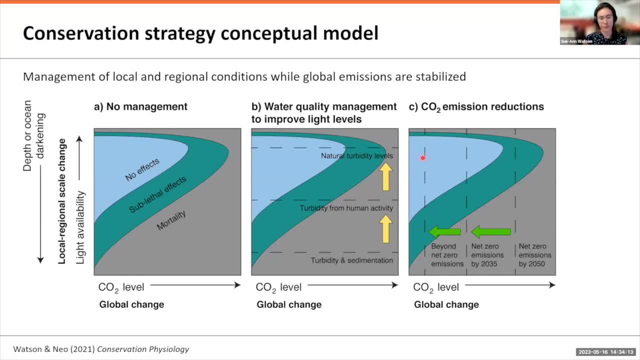 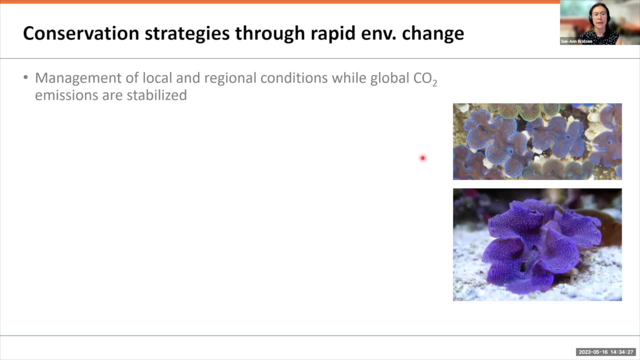 How we could sort of best position different factors that we could control, So local to regional and then global- to create that sort of safe space for giant clams on our reefs. So we've talked about that first one. We also identified a few other options in the paper and they included adaptive population management. 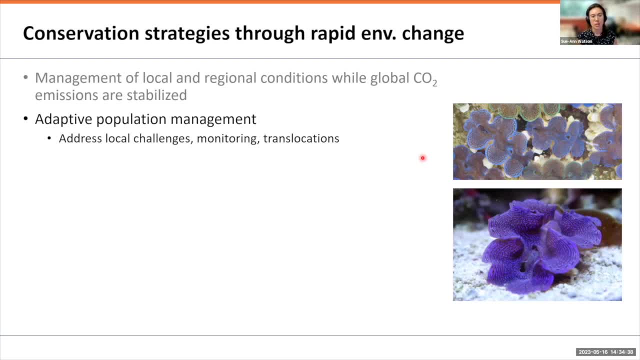 So, as well as addressing some of those local challenges that I mentioned, We could do monitoring more: monitoring of giant clams and during times of bleaching events and warm heat waves, As well as translocation of individuals from areas that are really getting hit by heat waves to other areas on the reef. 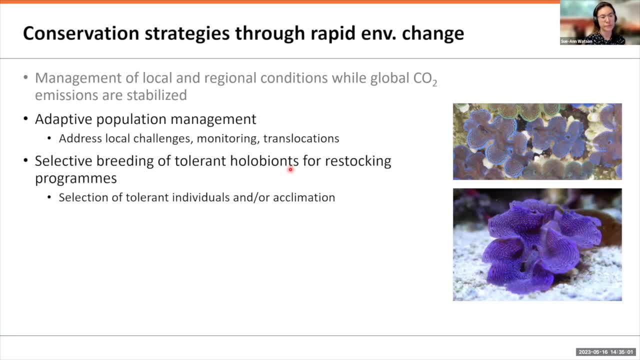 And perhaps to higher latitudes. We could also consider selective breeding of tolerant giant clam holocaust, So re-stocking programs, And so we could choose individuals that have been sort of tolerant to ocean heating conditions, Or, and we could get animals in an aquaculture setting and give them extra heat. 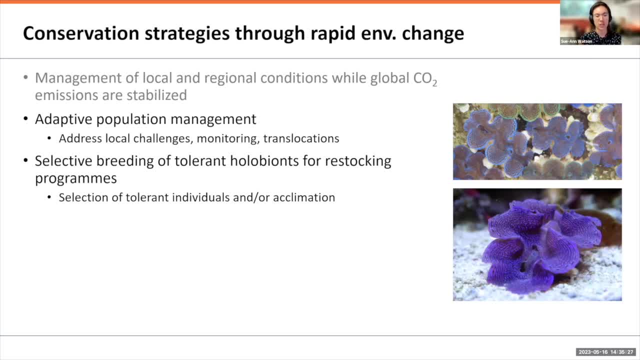 Either kind of chronically or a marine heat wave situation, And allow them to acclimate to those conditions And select individuals that adjust the best to those. Giant clams are not born with a symbiotic algae. They actually acquire it in early life. 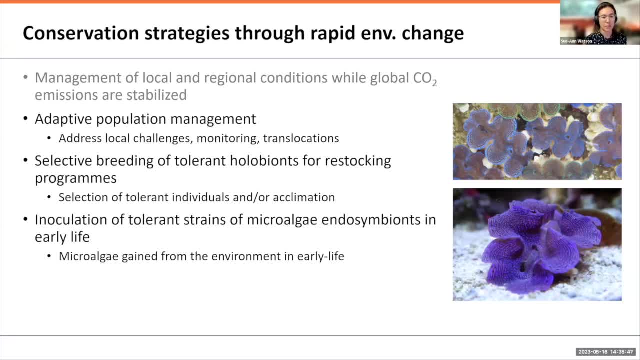 And so it's possible to introduce more tolerance change in microalgae to giant clams in that early life stage And so this could be a way to help with the rapid adaptation of giant clams as a whole, The whole animal. We also identified in the paper that we could try to value tourism potential more. 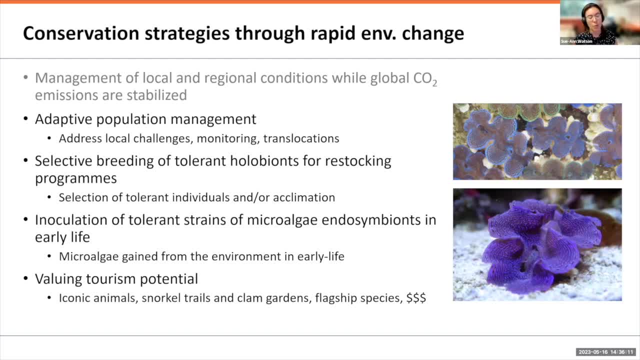 Since giant clams are iconic animals, We know that they're already used in snorkel trails and clam gardens. in certain areas, They could be considered a flagship species, And also if we try to value how much revenue is produced by tourists going to see giant clam individuals, 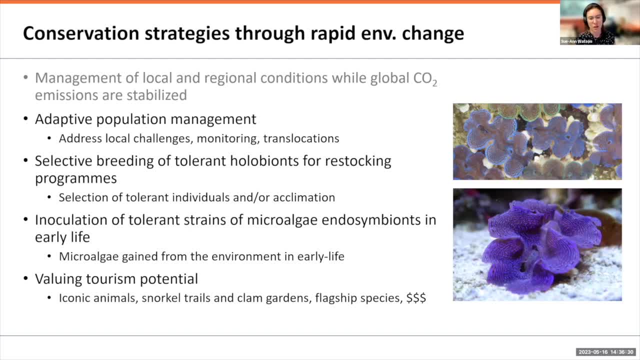 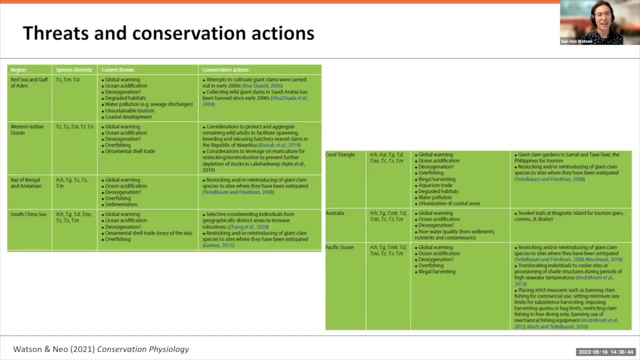 Then that might sort of incentivize the protection of giant clams as well, And people have done this with manta rays, for example. Now some of these ideas might sound a little bit far-fetched, But we actually went through and reviewed what was already being done. 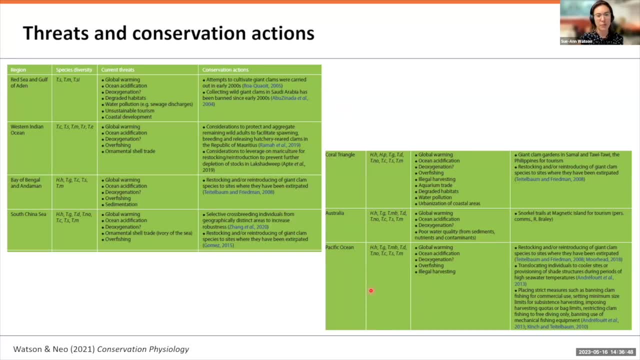 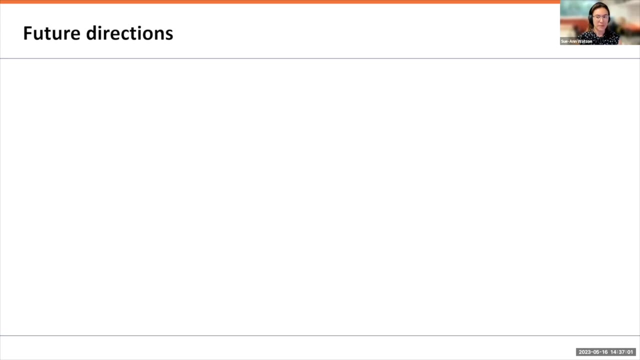 And this is a little bit of just a display from the table in the paper. If you're interested you can go and read that. But in some areas there are quite sort of active management plans For giant clams. Well, where to from here? 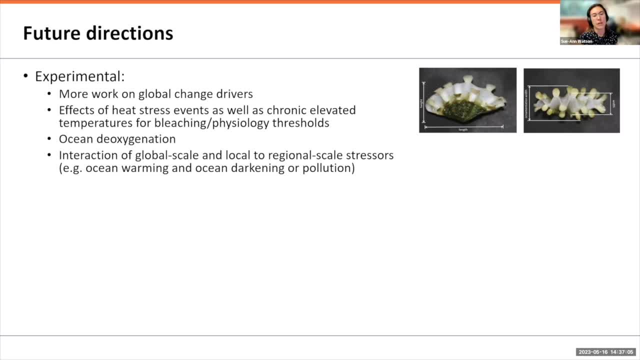 Well, we identified that we will need more experimental work on giant clams, More work on global change drivers, Understanding the effects for each of the species, More work on investigating heat stress events, As well as chronic elevated temperatures For any potential kind of bleaching or physiology thresholds. 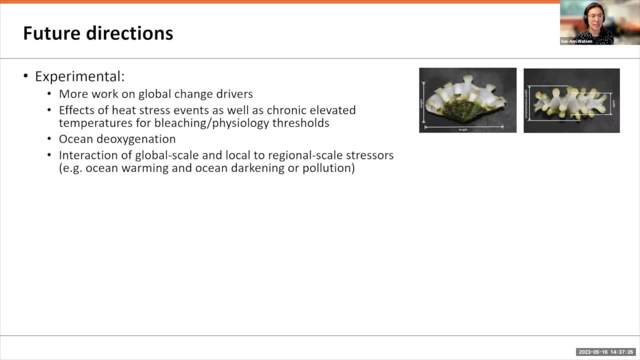 More work on oxygen and ocean deoxygenation. So a giant clam will evolve oxygen, But in the nighttime it draws down oxygen as a whole holobiont And overall there is a net take of oxygen. So we think that deoxygenation would be a problem. 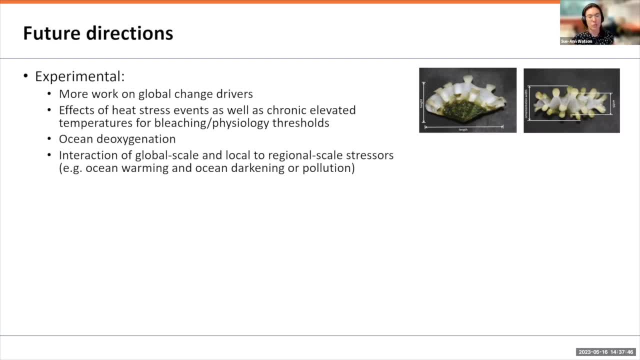 And the interaction of global scale to local, to regional self-stressors that have not yet been studied, Such as ocean warming And ocean darkening or pollution. Field observations are going to continue to be important, So field responses and monitoring of marine animals to environmental change. 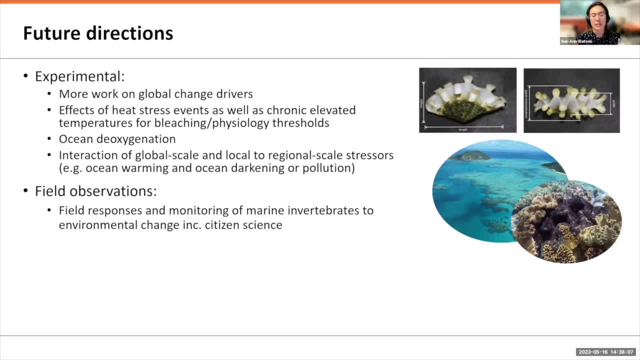 Including giant clams, And they really lend themselves to citizen science programs. So we're hoping there's an avenue there Which will also kind of increase public awareness of the problem. There's also death space work to be done, As I mentioned. 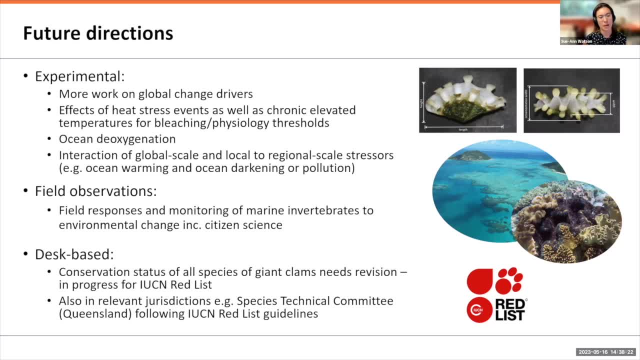 The conservation status of giant clam species needs to be updated, And this revision is in progress. Also, relevant areas could update or even include giant clams in their threatened species assessments, And this is something that I'm involved in In the species technical committee for Queensland. 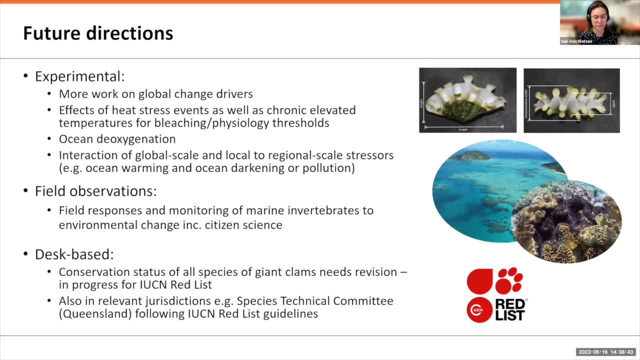 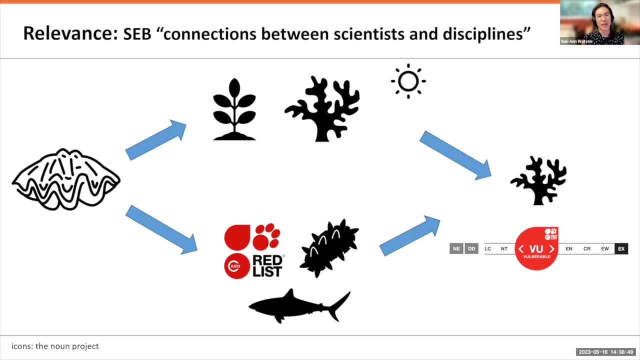 Where we follow the IUCN red list guidelines And then just drawing back to that figure at the start. So hopefully you've thought about some of the ways that some of the ideas and concepts that came out of our conservation physiology paper could maybe relate to your species or the ecosystems in which you work. 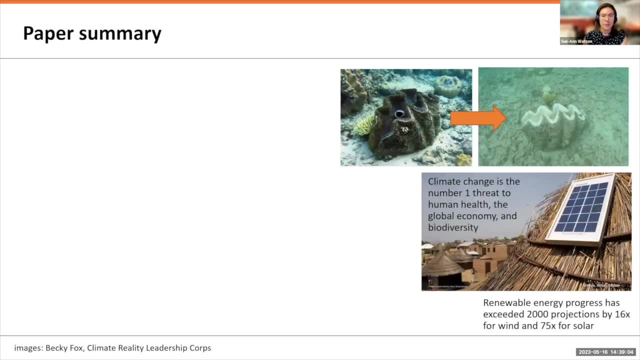 So, to summarise the paper, The primary problem here that giant clams face is global change And we urgently need to meet net zero greenhouse gas emissions as soon as possible And even really to progress beyond net zero greenhouse gas emissions to keep our coral reefs in that safe operating space. 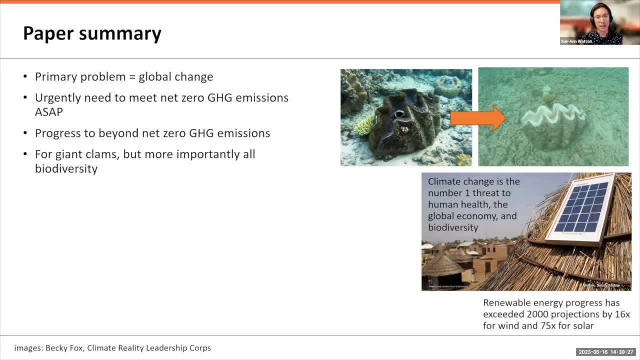 This is not only for giant clams but, more importantly, all biodiversity. We know that climate change is the number one threat to not only biodiversity, but human health and the global economy. Meanwhile, while we're getting to that- And we do have the great technology to get to, you know, clean, renewable energy. 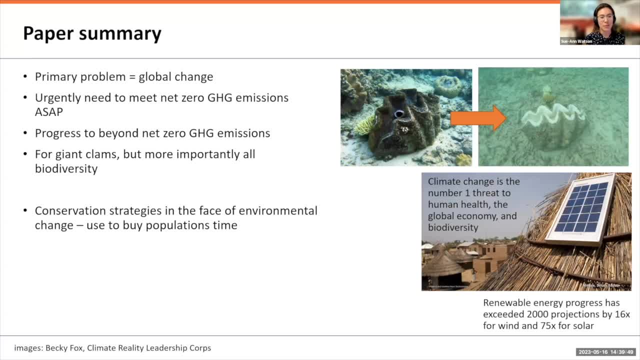 We need to focus on conservation strategies to buy populations of our threatened species, like giant clams, time in the face of such rapid environmental change. And we can see this because on coral reefs we're getting bleaching in these traditionally cooler La Nina years, So bleaching is becoming an annual event, which is really problematic. 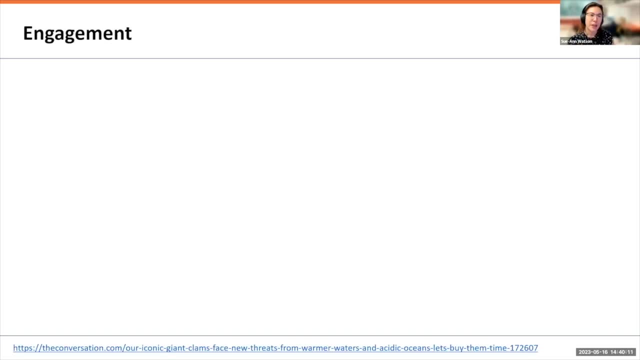 So what do we do after the paper in terms of engagement? Well, obviously, conservation physiology is open access, So that was really great in allowing accessibility for the actual published research for everyone. We also decided to buy a press release and an article. in the conversation, 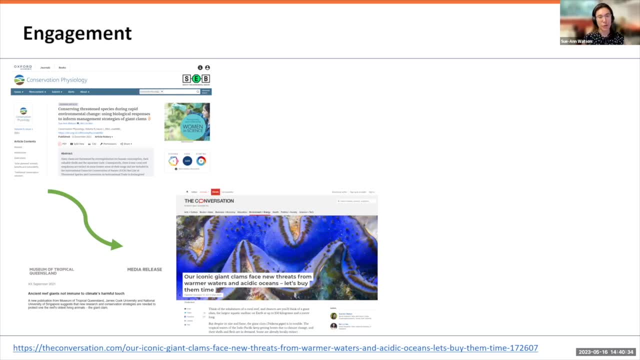 Now the conversation is an outlet in which you pitch your idea to And a professional editor will help you write your article, And this was really well received. It was a really good learning process. I would encourage everyone to have a go, And actually it was just after one of those IPCC kind of COP meetings. 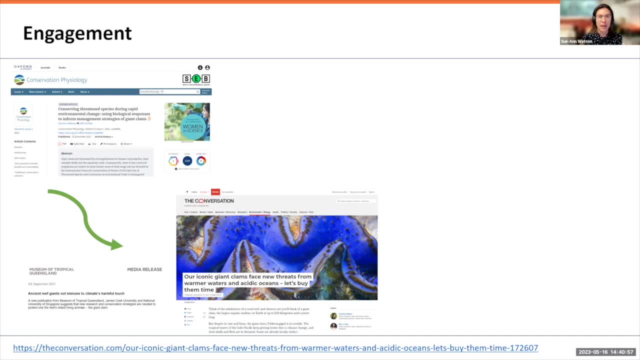 And we had a lot of sort of uptake from the work. It went out as the lead article for the day. So the media release And then that sort of public accessible article was really good in helping to get the word out about the paper. 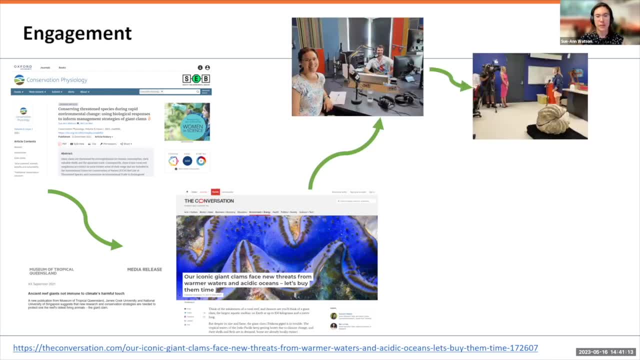 I also did sort of radio interviews. We did a bit of TV. There's the giant clown specimen that we have in the museum out on display. That led to some national radio interviews And it also led to an international Pacific beach radio interview. 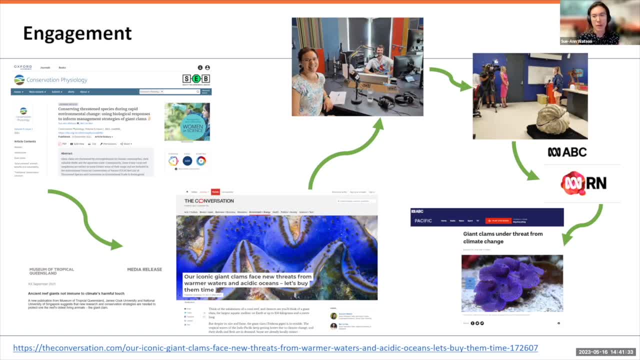 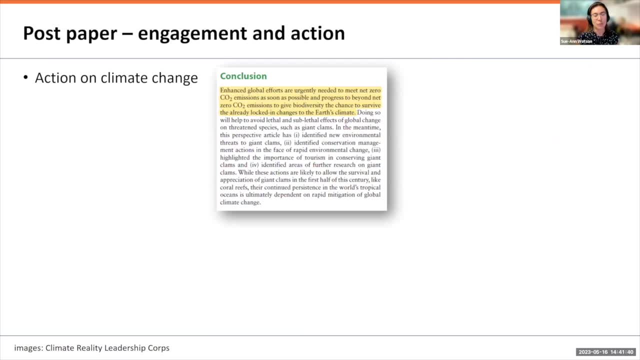 So that was really good engagement for that paper. So, post paper. what have we been up to? Well, again, I guess sort of just the action on getting the word out about really acting on climate change, And we had put some of that in the end of the paper. 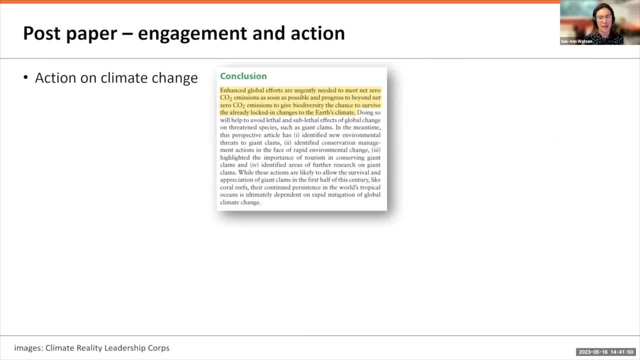 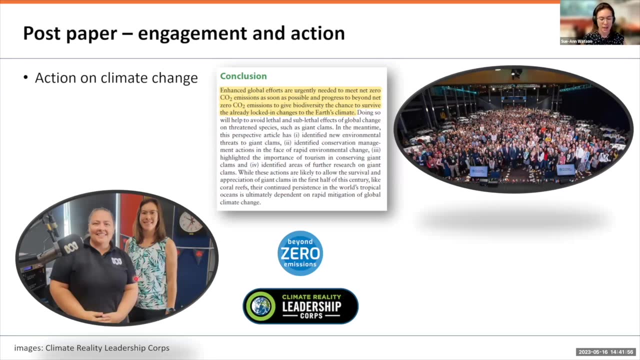 So that was sort of quite a nice message to continue to get out there, And so that's things like more radio interviews. This is the one that I did last week. We'll also continue to get more interviews. So strategic new collections and collection research for our threatened species, including giant clams.